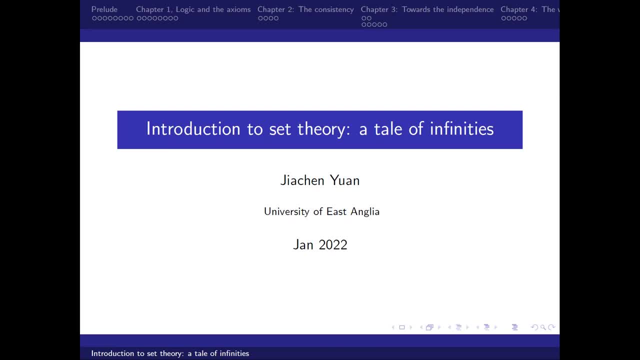 Dr Teo. His PhD thesis is about precretite forcings and models of ZF and his research interest is on set theory and pure model theory. So today we begin the first lecture by Dr Yuan today. So, yeah, I guess I can pass it on to you, So go ahead. 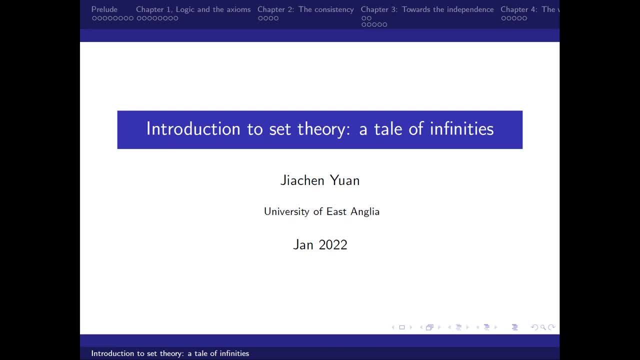 Okay, thank you very much. Thank you everyone for waiting with me till so late. Okay, I'm going to give a very general introduction to the infinities, without running into details. I hope all of you can follow me. Okay, it's just a pause for a moment. 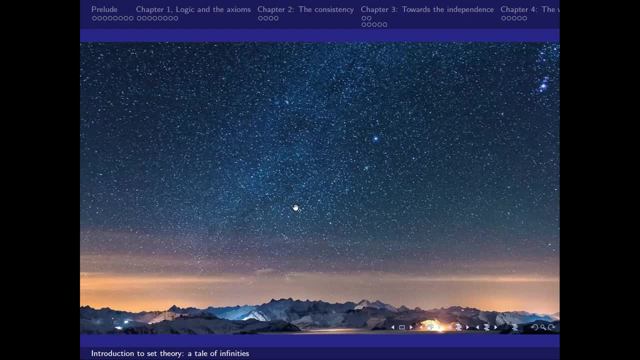 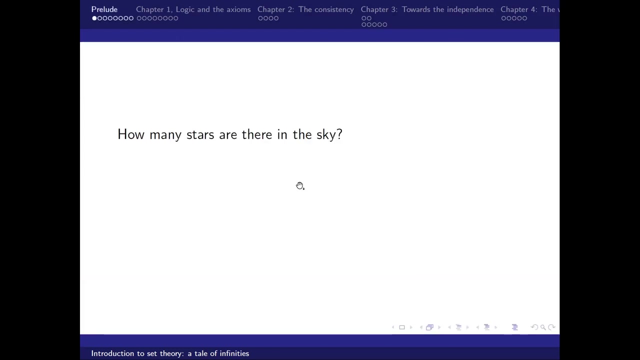 So I think, let me So when we were, when we were kids, when we are looking up into the night sky, when we're wondering how many, how many stars are there in the sky, So we may start count, number The number of the stars: one, two, three. 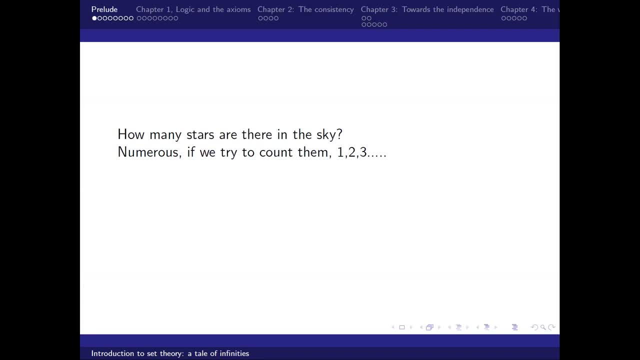 Okay, but now let's just use Our imaginary power to jump out of the physical world. just continue counting process one, two, three. It looks like for us this process can go forever. So that's how we perceive the concept of infinite. 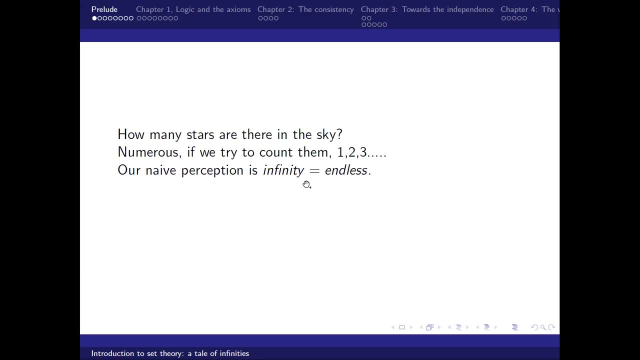 That's the first place. So Our very naive perception is that infinity is just some unblissing, or at least it's just as what I said, how it looks like in the first appearance. So if we just stop here, infinity is just the infinity. 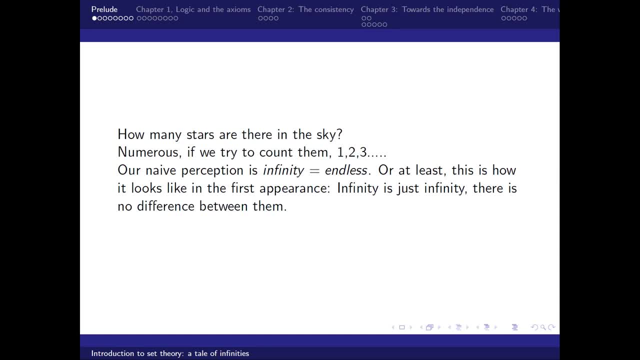 There's no difference between them. But is that true? So all right, indeed, there are different infinite states. for instance, we have the set of all nature numbers, the set of all odd numbers, the set of all even numbers and the set of all prime numbers. 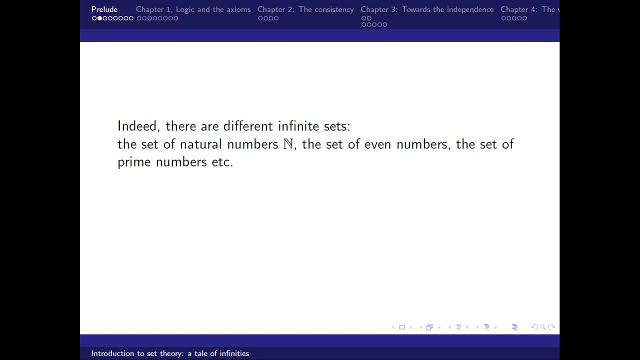 There are different infinite sets, But in terms of how to Count them as a really different infinities We are. the reality is not. they are actually the same infinity. Because you can, let's say we can- just recount The set of prime numbers. 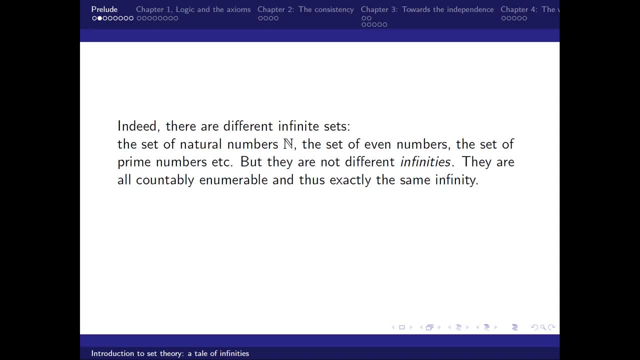 Exactly The same way as we count natural numbers. we say that the first prime number is two, as the second prime number is three, so forth. i mean, it's just dependent on the way that we count them. they are just the of the same cardinality: the set of all natural numbers and the set of all prime numbers. 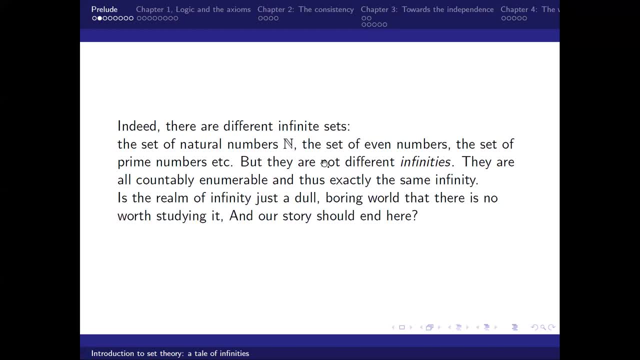 so we just wonder if the the realm of infinity is just a dial boring world, namely it's just a trivial, there's no difference between the infinite sets. then we can just stop here, everything just. we just end this talk. but you can see the slides there are. 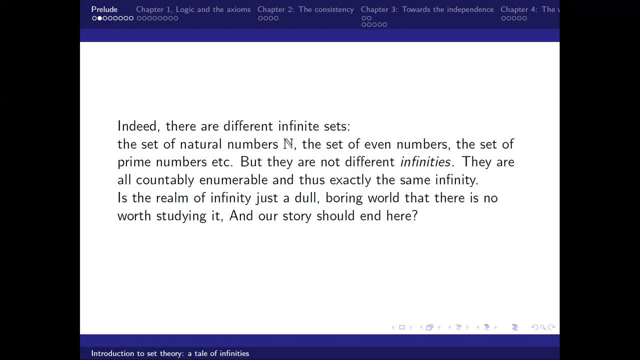 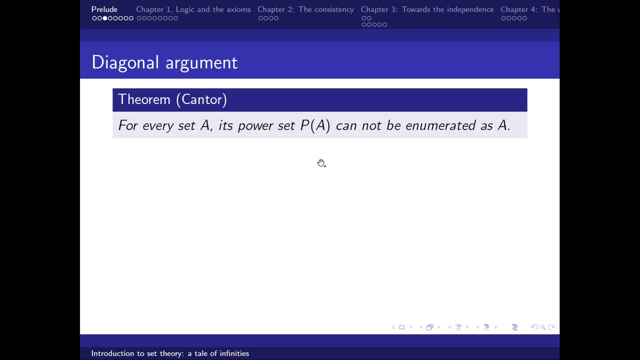 a lot of slides afterwards, so it's not so interesting. reality, okay, the first significant observation is by canter. he proves that for every set, essentially its power set is not the same as itself regarding to the, the number, the size of it. so here is his proof. 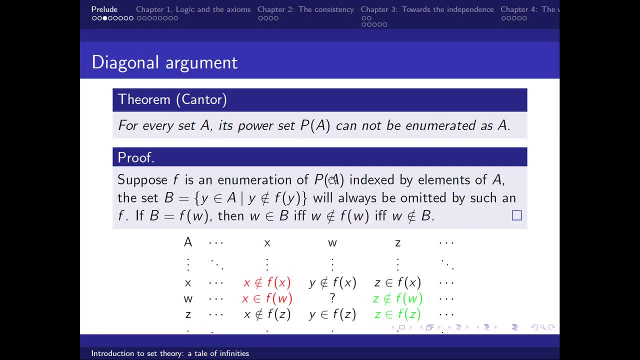 so suppose you can enumerate the power set of a as a, so you can see. i threw a picture below. so the vertex line is just the numbers of a, the, yeah, the members of a, and we are going to the horizontal i correspond to. each member is just the. 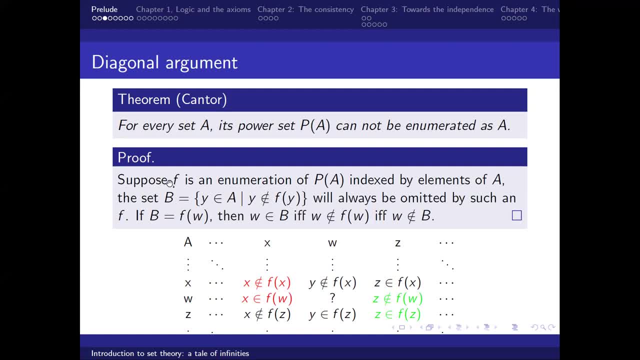 the set, which is correspond, corresponded by a. so how about the diagonal element of this diagram? so let's say b is a set, so that y is in a but y is not in a. y, so let's just suppose a- it's obviously a subset of a- is enumerated by f. that's what we have assumed. 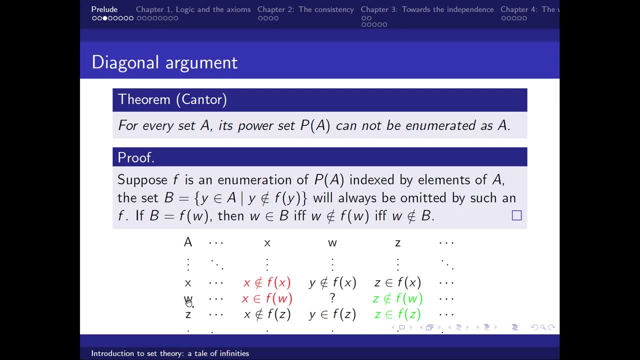 so let's say it's fw, so w is here. so what we can say about such a b? so let's say we ask if x is in fw or not. so x is in fw, if only if x is in b. by definition, x is not in f of x. so okay, x is in fw, all right. 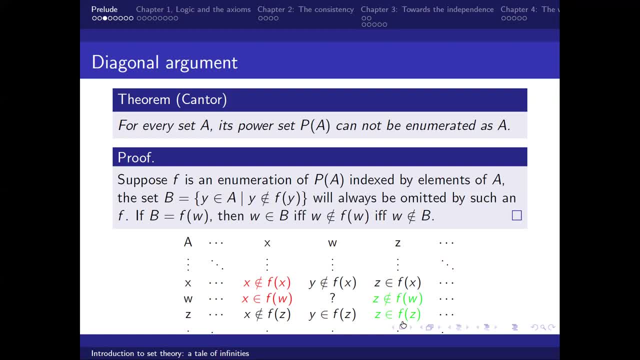 how about z? so if z is in fz then by definition again, z is not in b, namely z is not in fw. but there is going to be a problem when we consider the element w. so let's say whether or not w is in b. so let's suppose w is in b, then w is in f of w. 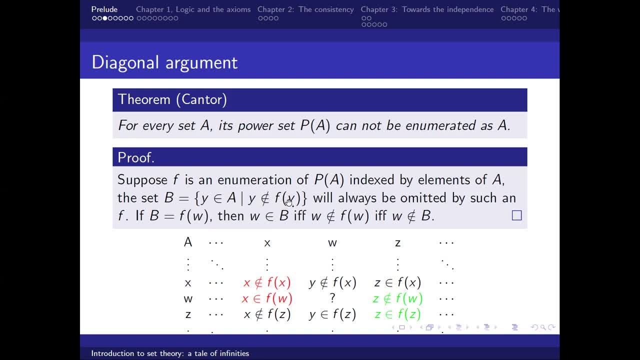 but by definition here the definition of b, w is not in f of w, but f of w is rb, so w is not in b. so if we start with w is not in b, then the same thing, i mean the proof, just go this direction successfully again. so it, i mean there is no. 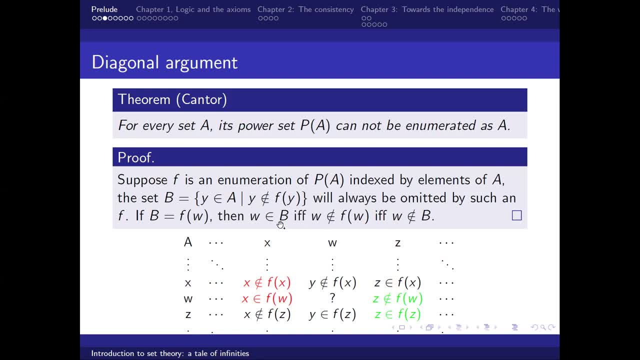 answer to w is in b or not. so thus it's a contradiction. the contradiction comes comes from that b is enumerated in this diagram, so, which is not possible. this gives us that the power set of a is not, can never be enumerated, enumerated as a. so there are indeed in, there are indeed different infinities. 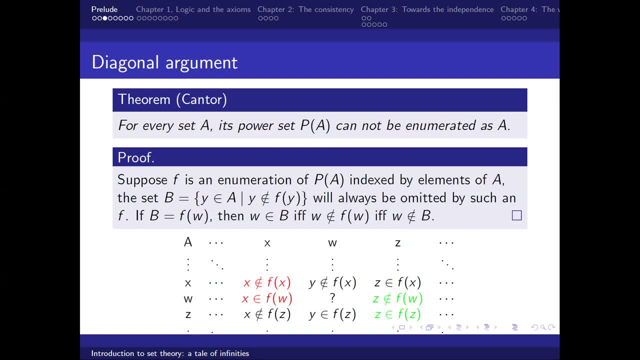 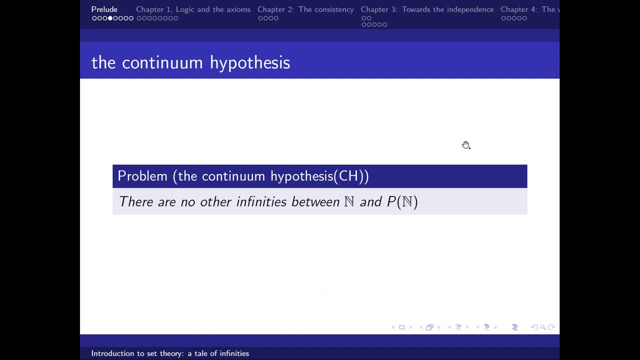 like for any set, a, its power set will have different size of a. okay later on after this. so the realm of infinities is not boring. it's not always, and at least it's not trivial, but how non-trivial it is. so let's say, let's take a look at our first infinite sets, the set of natural numbers. 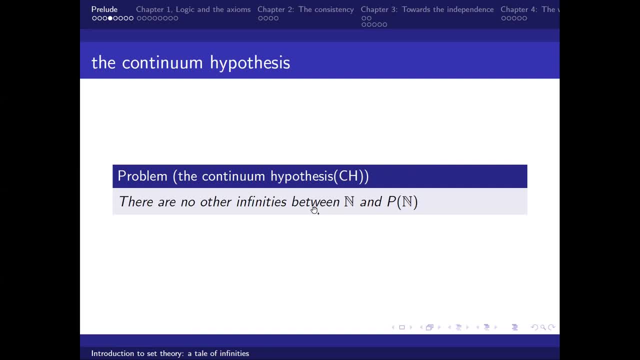 so are there any other infinities between the natural number at the power set of it? that's- uh, that's called the continuous set. so let's take a look at the continuous hypothesis. it says there's no infinity between the countable set and the power set of the countable set. 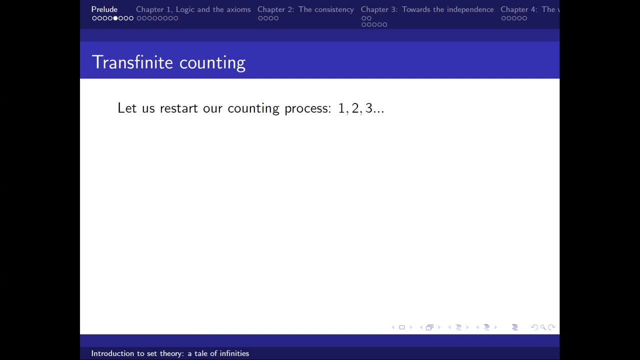 okay, let's just move away from this a bit. so let's just go back to our counting process. so one, two, three, but this time let's just imagine our endless process. just n at some point. so let's just collect all the natural numbers, the set of natural number. 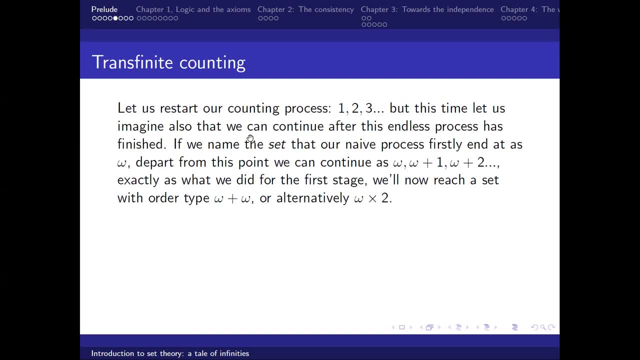 so let me call that omega. and from that omega we keep adding successor element to it. so let me call that omega, and from that omega we keep adding successor element to it. so let me call that omega, and from that omega we keep adding successor element to it. 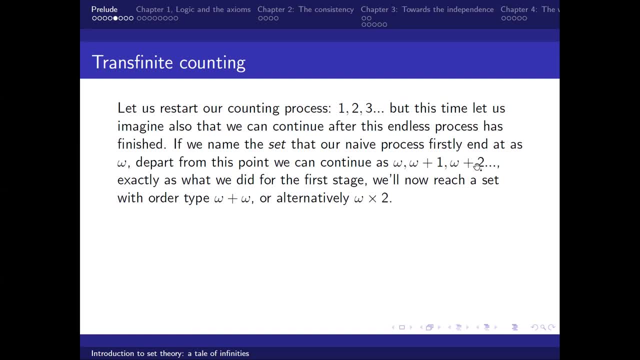 like omega, from omega n, omega plus one, omega plus two, etc. then we will reach the sixth limit stage, which is of order type omega plus omega, or alternatively we call that omega times two, so forth. we can reach omega times three, omega times four, et cetera. 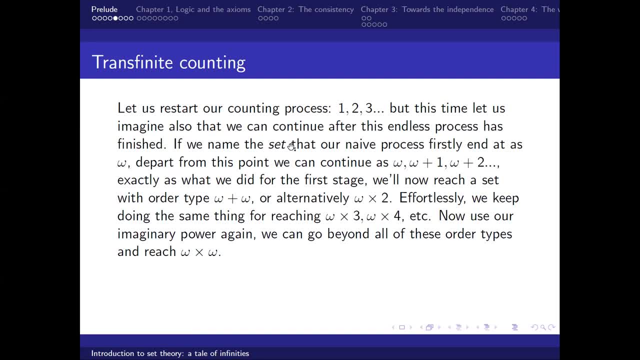 Now we can imagine this process is not finished, So we end up somewhere. but we just take the set for gravity So we can reach without any effort to omega, times omega. So let me show you, if I can draw a picture to show you, how this goes intuitively. 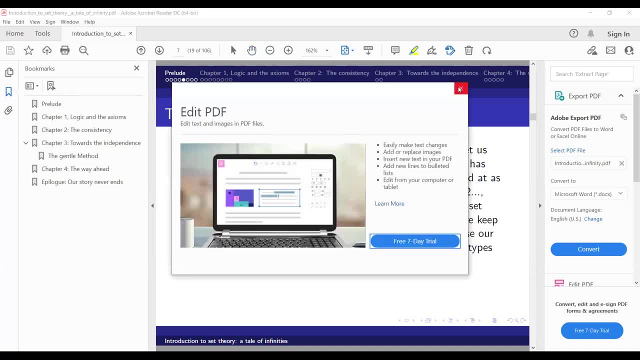 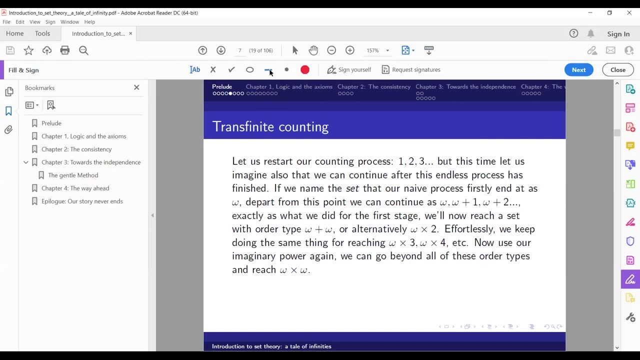 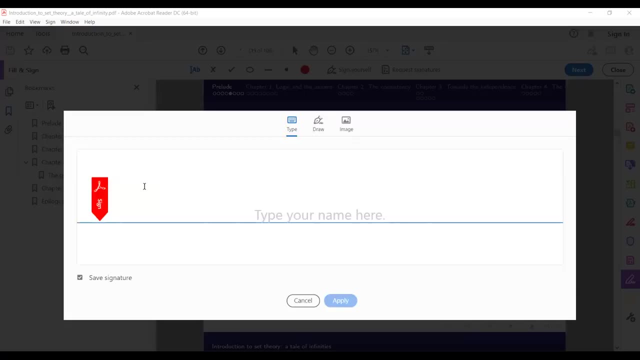 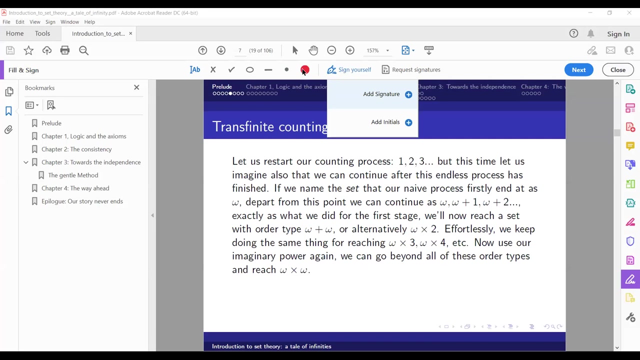 So let me see, Do you know how can I draw something here? Okay, okay, That's good. So let's just try to say how this process goes. So this is one and this is the order. type two: add one more three. 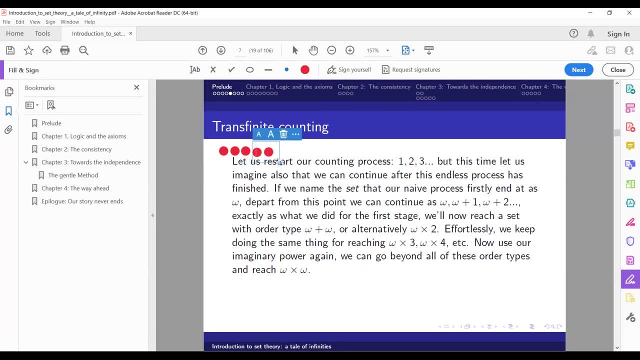 so forth. Okay, let me make that smaller. We don't have enough space, Okay. So this whole thing, this infinite process, is going to end up with something, with a limit point. Let's see here Is it? I'm not good at this. 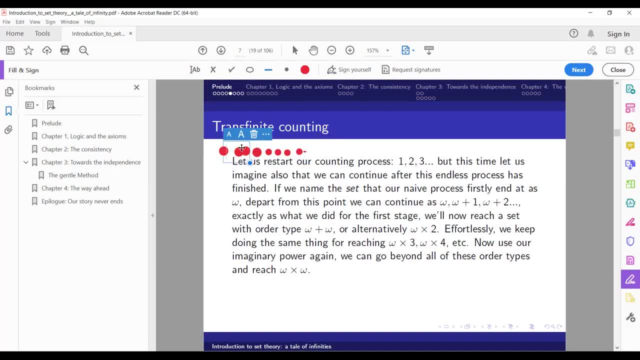 Okay, So this is the order type. So this is the order type omega, And from then on you can keep adding successor to that. So this is the first limit plus one element. So this is omega plus one, plus two, plus three, so forth. 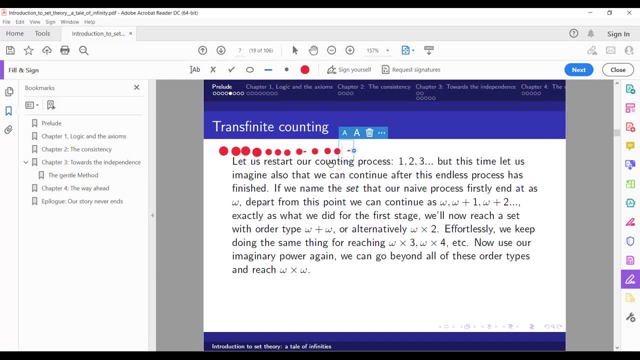 Then the same limit plus one plus two plus three, so forth. Then the same limit plus one plus two plus three, so forth. Then the same limit, exactly. copy the first process. We've reached the order. type of omega times two. 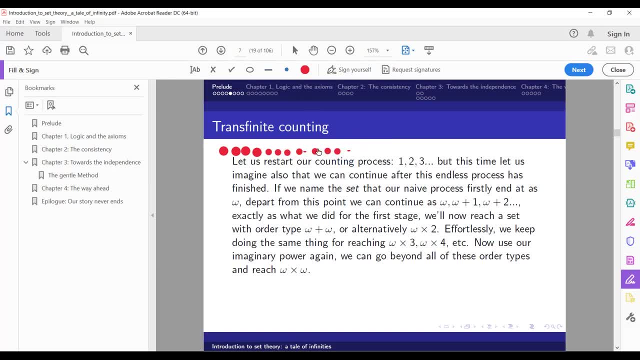 So you're using the dash to represent omega, right? No, no, I'm just. the dash is just the endless thing. The oh, it's like the same as the. Okay, I get it. Okay, yeah, Okay, it's just the. 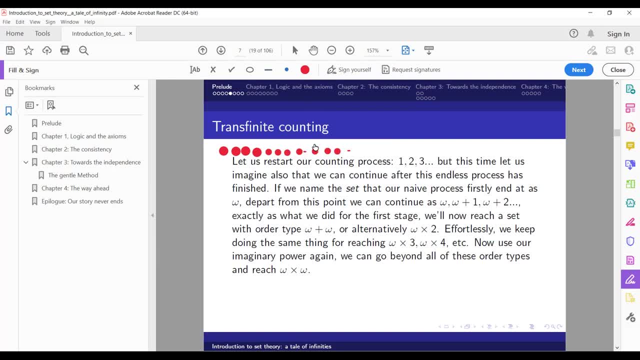 because I cannot, I don't have infinite time to show you. because I cannot, I don't have infinite time to show you. Okay, I get it, Okay, yeah, Okay, it's just the because I cannot, I don't have infinite time to show you. 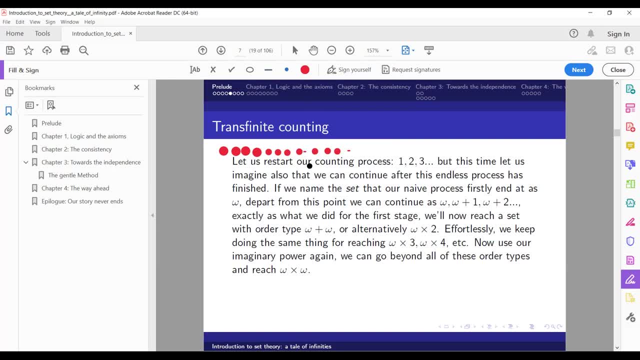 Okay, I get it. Okay, it's just the, because I cannot, I don't have infinite time to show you the infinite processes. You just imagine that I, in some time space, I draw infinite many dots here. Okay. 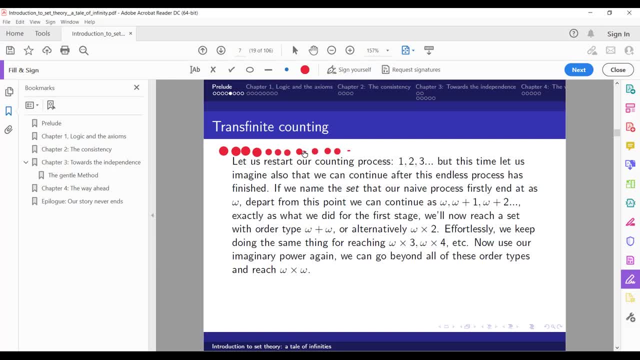 But we jump out of that universe. we can see the whole process. Do you get me? Yes, yes, So, but okay, so this is omega times two, so force omega times three, But if you will, the, the state, the. let me just add the. 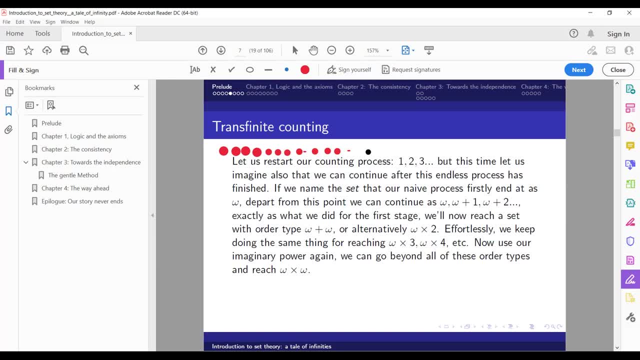 But if you will the, the state, the, let me just add the. But if you will the, the state, the, let me just add the. so let's just name the first big state as the first the infinite many states. 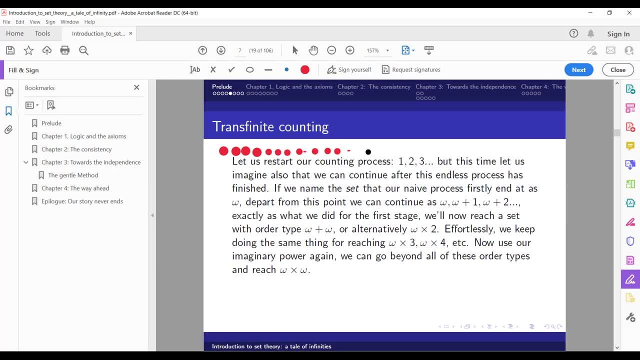 So, instead of adding one element at a time, we add omega at a time. So the same. So the same, because the same infinite hurry process just gives you the omega times, omega, right. So you, just you, kept going, but you kept going for infinite minute times. 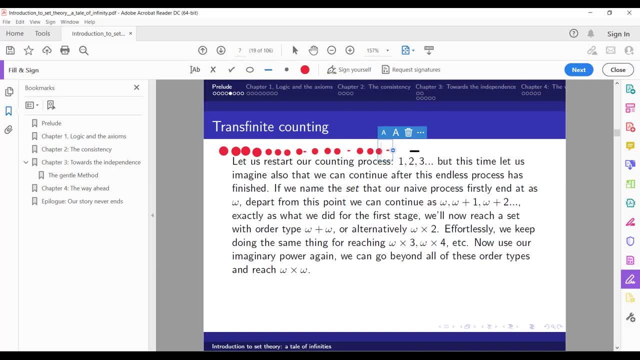 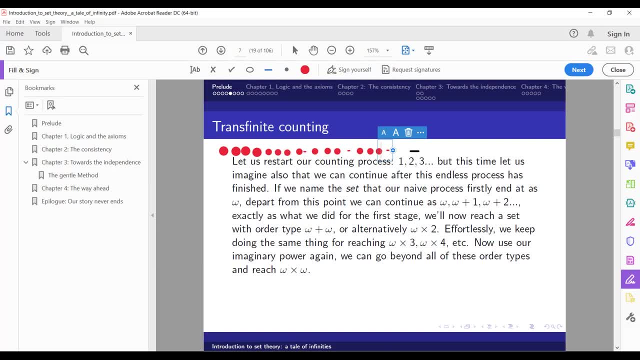 So just imagine, whenever you have a process you keep going but it will reach a limit because you can only take finitary states to that. But you can imagine that can go forever, But once it's finished, I mean you just jump out of that time space. 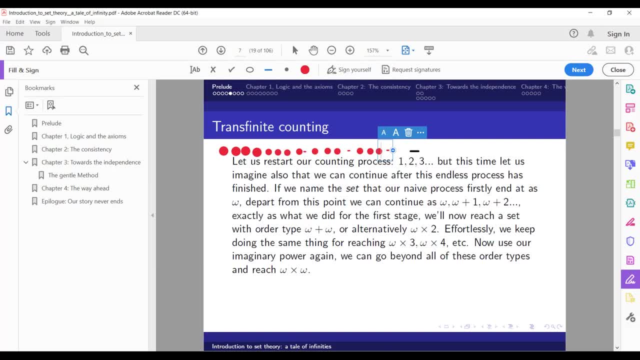 You can view the whole object. Oh, then you realize, yes, we can go to the next state. So I don't know if you get me or not. Should I assume you are fine still following me? I think it should be okay. 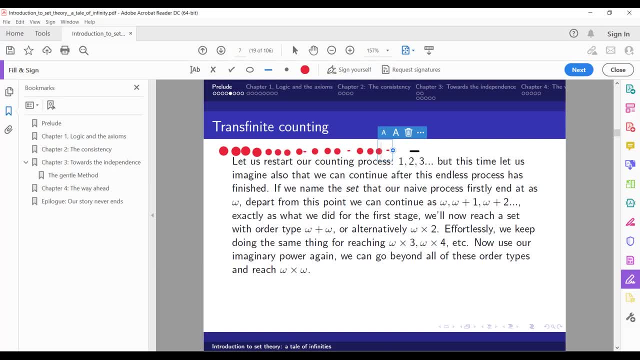 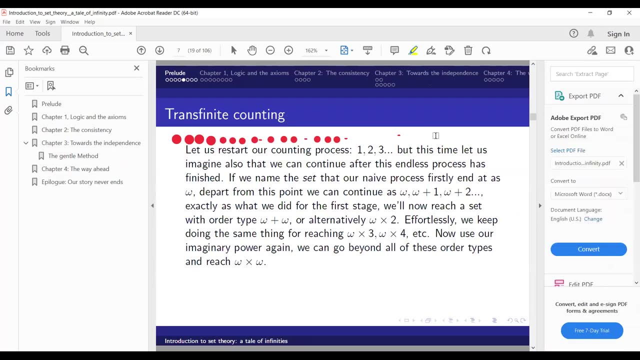 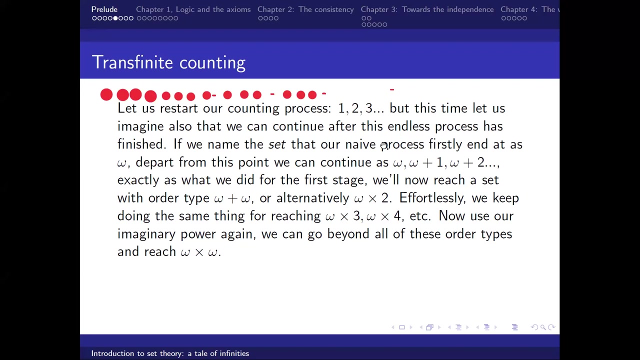 If anyone has a question, you can let us know or you can type it in the chat, But so far no question yet. So I think it's okay. Okay, this is a transfinite country, But we have to be careful about how to use. 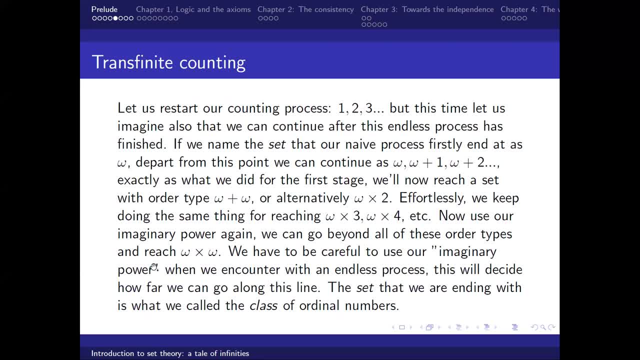 our imaginary power, like how we jump out of the universe, Because I mean it's kind of paradoxical if we say that we end up with somewhere but we just jump out of that time space to keep counting forever, But this whole thing. I mean we are leaving one timeline. 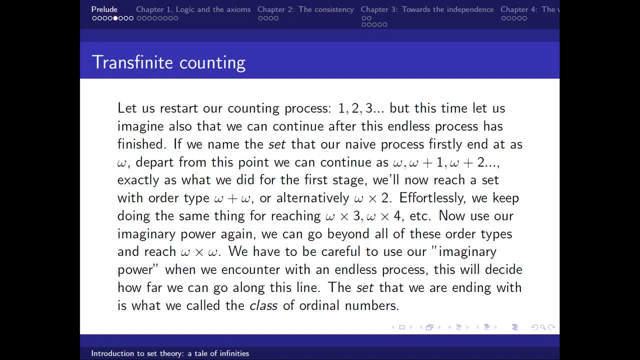 So there is the end of this whole thing. So where it is, it's just the strength of our axioms can tell. So the sets that we are finally end up with is what we call the class of all the numbers. But how many of them? 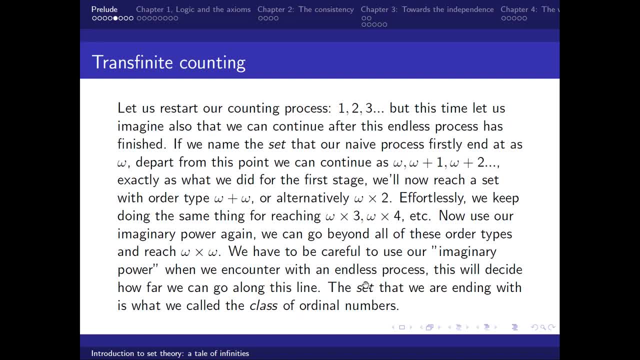 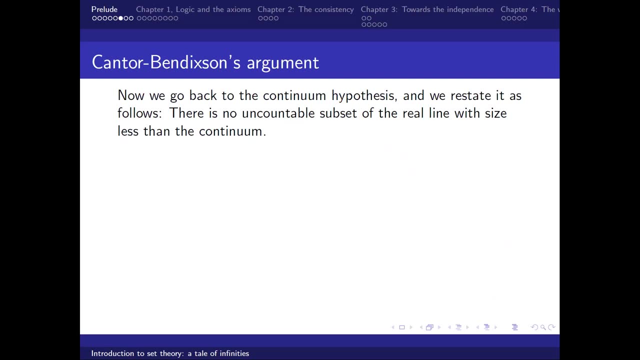 only the axioms can tell. I will show you a little bit more later about this, after I just gave you the axioms. So okay, let's just move back to the continuum hypothesis. So there is a way to restate it. 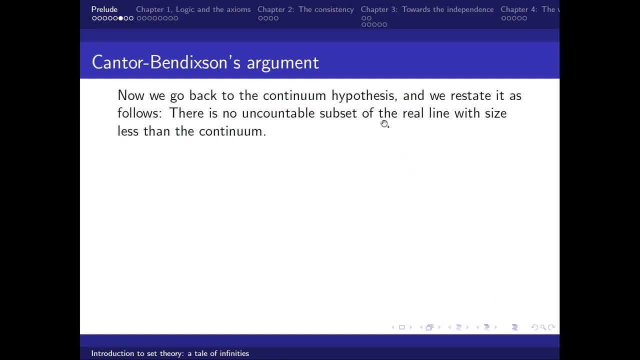 So it says that there's no uncountable subset of real line with size less than continuum. So there is a standard way to view the power set of natural number as the real line. So it's just a reformulation. Oh, okay. 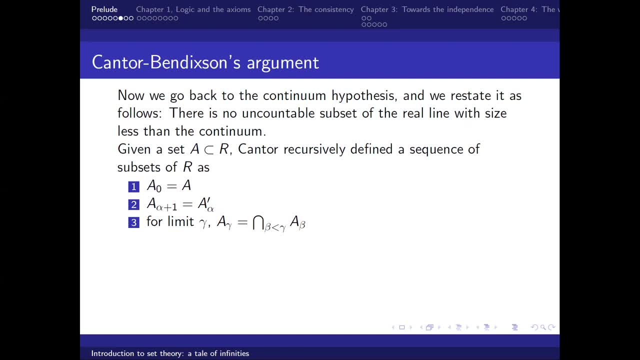 Cantor introduced the way to analyze the subsets of R by taking its limit point. Okay, And the following theorem says that the sum of all the values at a set in s of thepha, alpha and alpha should be the sum of all the values of S and A. 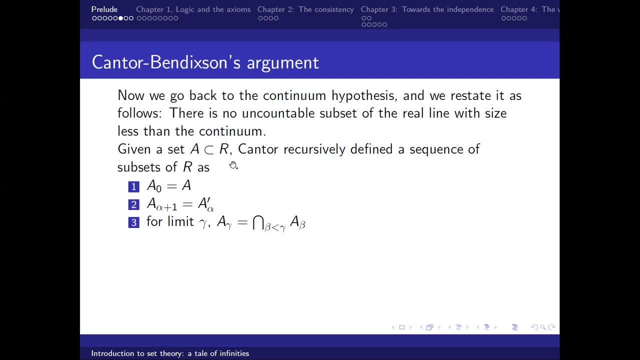 So with that, let's try to find the expression for lips. So let's try to find a deposition ratio of a set to two values of the first of a set. Let's try this. Let's say global win range. here is one matrix. 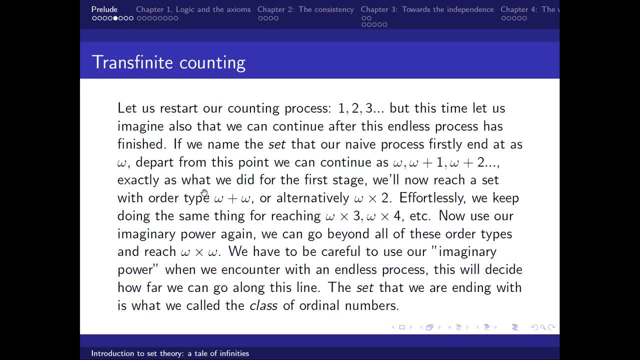 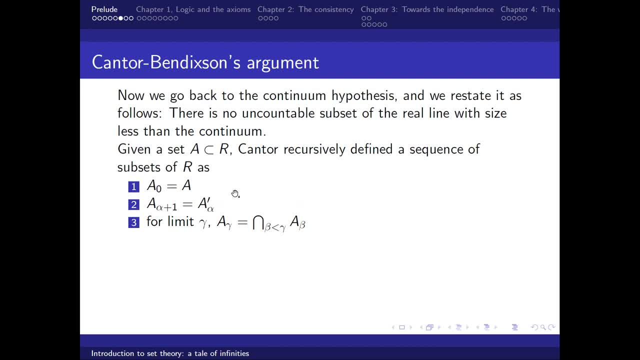 And if there's a lot of zeta, there should be a general distance here, And if there is a limit, there should be a maximum set. So let's try this, I will show you, Let's try this. So A alpha plus one is just the limit points of A in the sense of the topology of R. 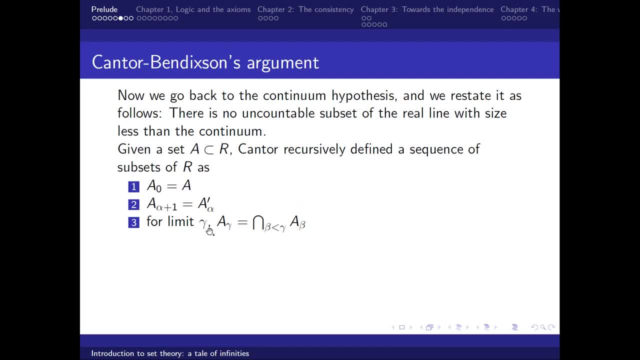 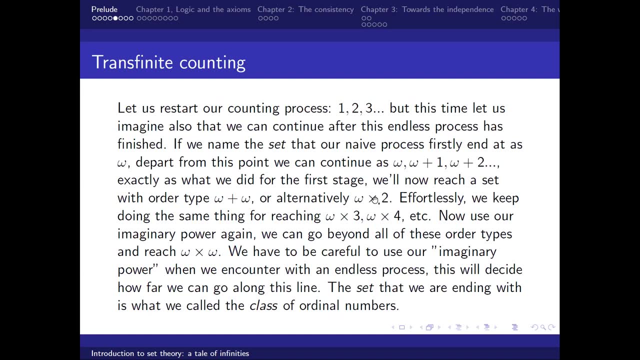 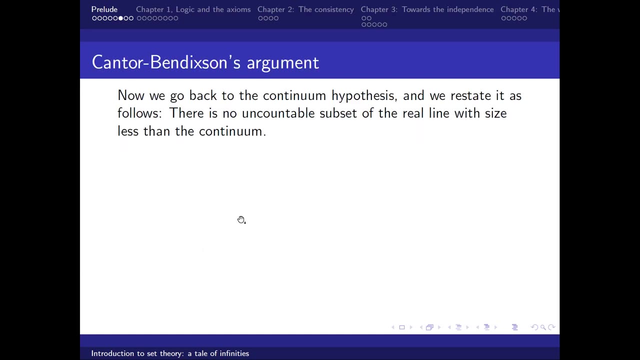 And for limit gamma, for instance, R omega, R omega cross. two omega cross, three omega cross omega. if gamma is this, cardinals, if gamma is this kind of cardinals, then you just take the intersection of all previous sets. 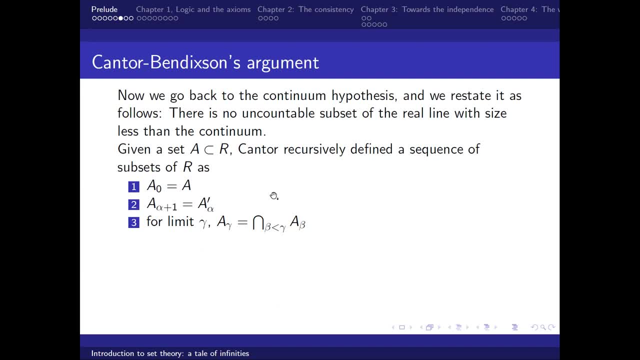 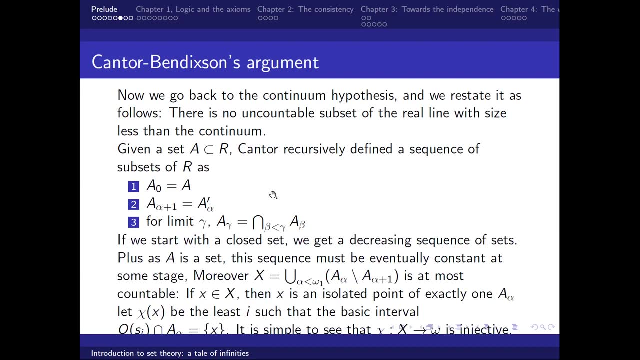 OK, this is the operation that Cantor used to treat the sets, especially for closed sets. So if we start with a closed set, so we are going to generate a decreasing sequence of sets, Because for a closed set its limit point is just in that set. 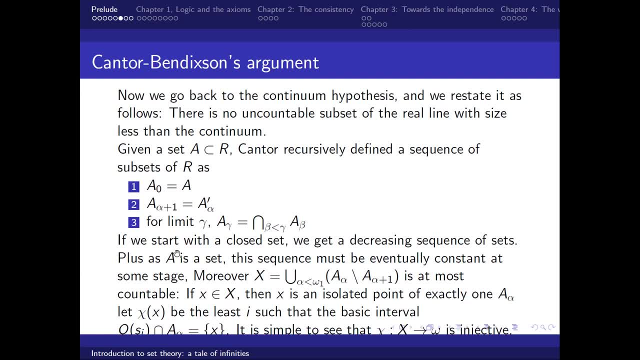 OK, So also A is a set. So this I mean you get strictly smaller and smaller sets, But it must be eventually constant, because I mean it has a size of sets It cannot, can never be matched up with the ordinal line. 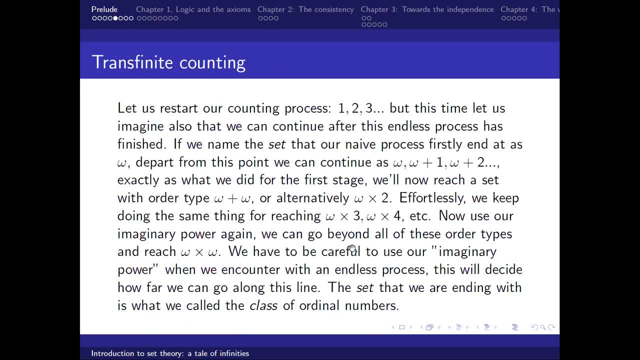 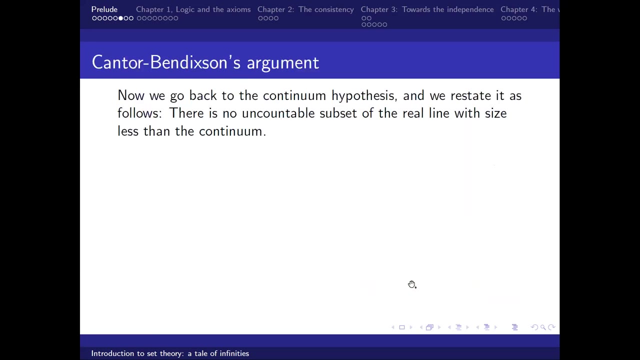 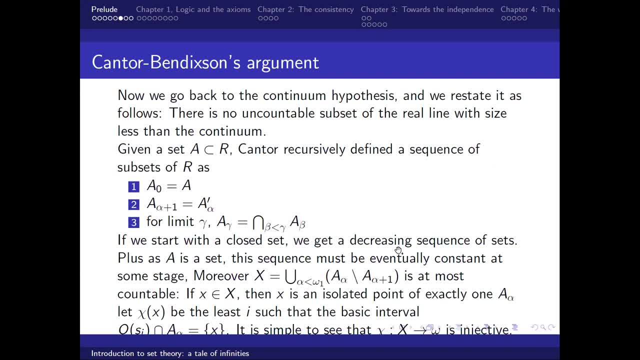 of replacements. So OK, So it's going to be eventually constant, Right, Right, constant. Moreover, we can just take a look at the union of the sets that we have removed from the original set A Now. remember that A is a closed set. 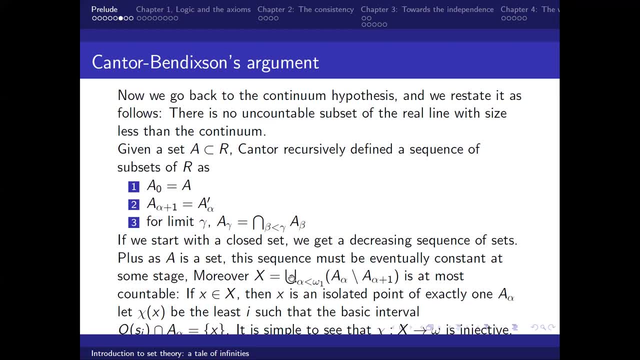 So this set must be countable, Why? Because if X is a element of X, then X is an isolated point of exactly one, A alpha, And there is going to be a basic open set which gives you that it has the only intersection. 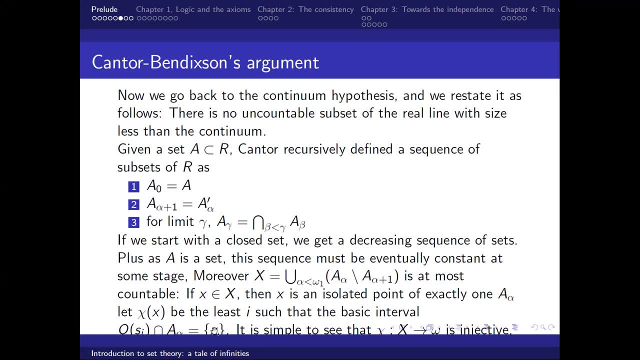 of A alpha as the singleton X At this chi you can map such X to the coding of the X. So this is the basic open sets, but they are unaccountable, meaning basic open sets. So R is second countable. 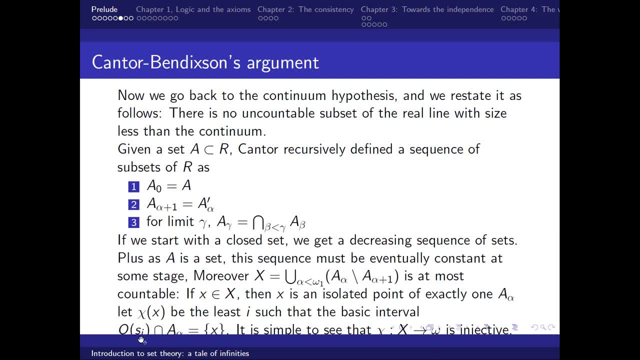 or I mean there is a standard way to define the basic open sets. So then it will inject the set X into the set of natural numbers. As I said, this set, finally, is countable, So are you okay with it? Okay, let's move on. 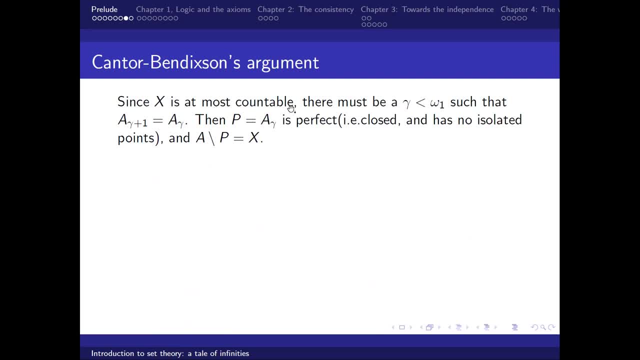 So, since the X is at most countable, there must be a set, A alpha, So there must be a countable ordinal so that it's start to leveling off, start to level off. But then if you look at such a set, 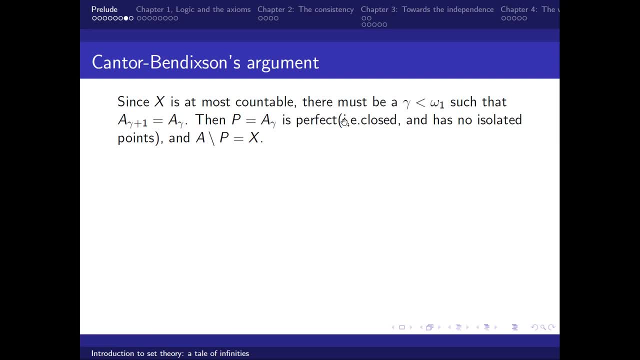 it's going to be a perfect set, or namely closed, and it has no isolated points. Because if it's once it has isolated points, then A gamma plus Y is not going to be the same as A gamma. That's what you say here, right? 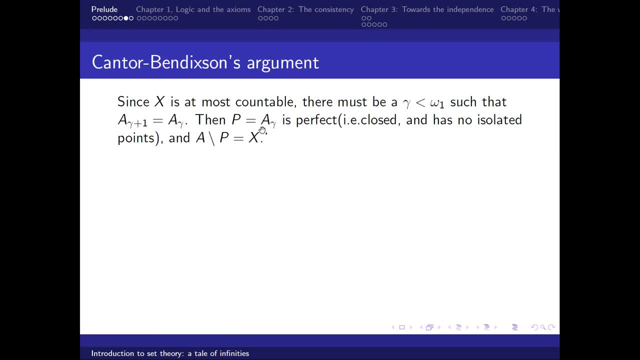 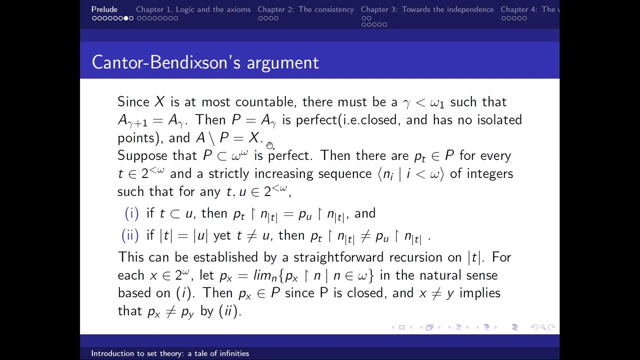 So its kernel A, gamma, is a perfect set, As the difference between the original set A and its kernel P is just the accountable set X. So the difference between the original set A and its kernel P is not going to be the same as the actual set P. 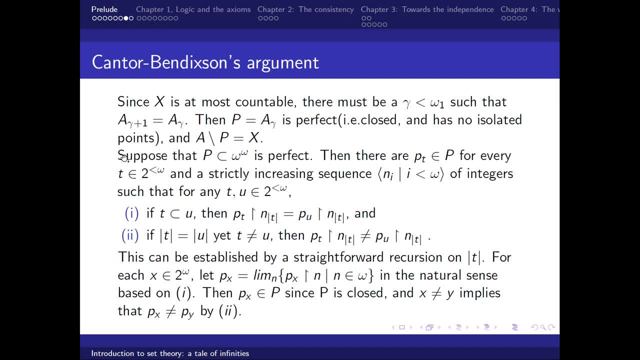 Okay, let's just do a bit study on the perfect set. Despite it's a paragraph with a lot of things, but I want you to have something in mind: that this process is just going to be similar to the construction of the counter-meter-third set. 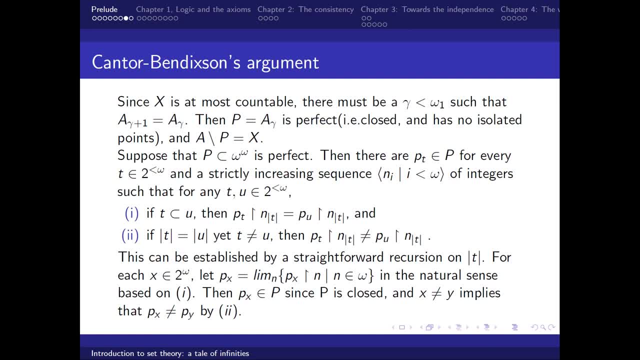 So it's basically this whole paragraph is going to show that any perfect set is going to be of the same size as the continuum. So you start with the set and you are going to build through the index and the two-to-late set: omega. 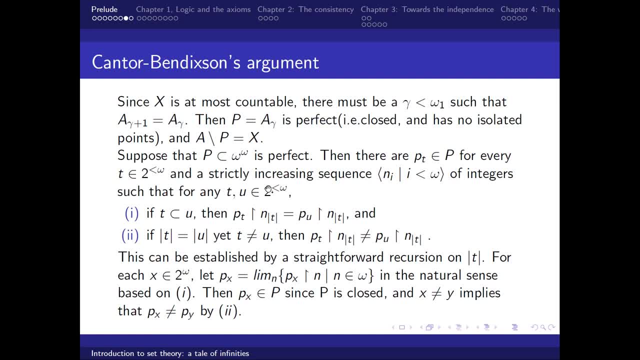 But you separate at each stage exactly what one and two tells you. So you build through the indices along this tree on two-to-late set, omega, but you get smaller and smaller and you narrow down the set by this hugeання. 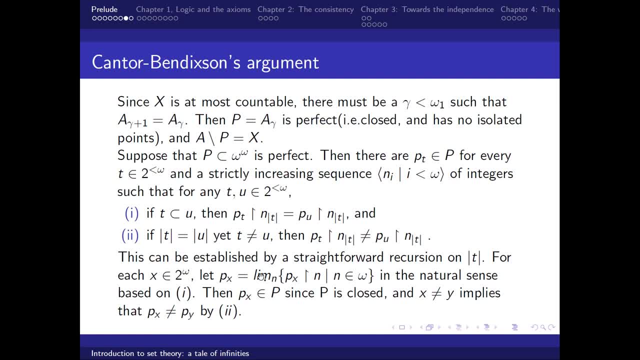 So you just go from this first two-to-late set頂 to this next two-to-late set and this little Wah of this form struggle first half. So on the third you do the fouling LP pulls for the first 5 here. 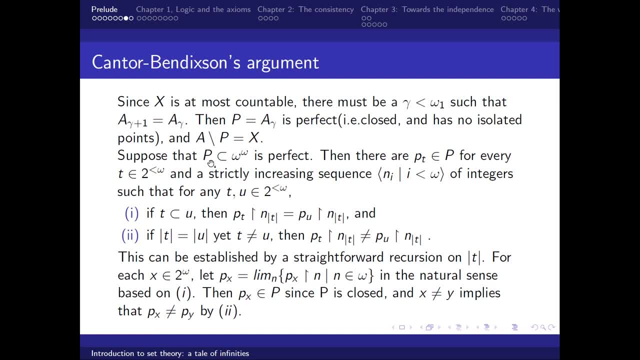 and for the next 5 you do a pull up and disperse the set and broadcast the curve to the one-to-last set again. That's how you decode a set. we call this minute set. All right, so before we go into, 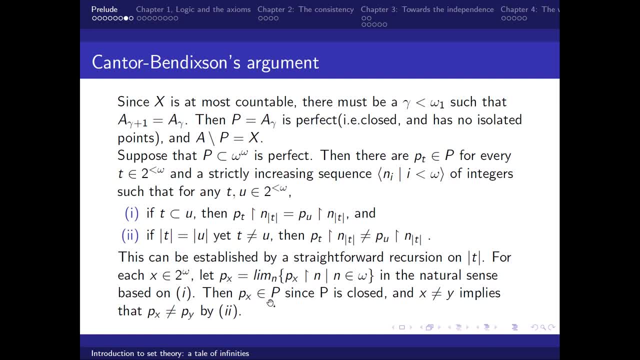 give you an element px in p. So this paragraph is going to give you a way to show that two, two omega is just the injective into such a p, At last. it's the perfect set is always large. It's the same size as the continuum. 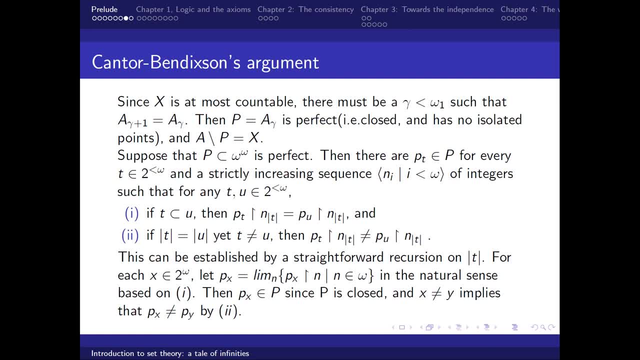 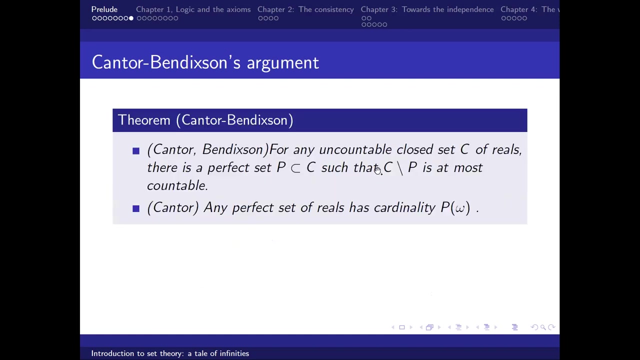 So is everyone okay with this? Or you want me to pause for a moment, then you can read through the details, But I mean, it's just the same thing about the counter mid start construction, So I just move on. So this is what Kanto has established. 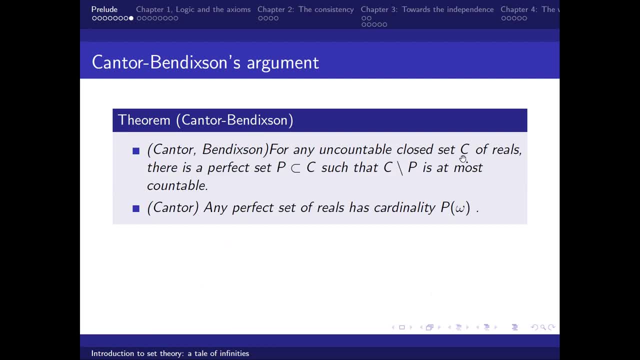 So for Ariane, uncountable close the subset of rails. At least it has perfect set product. That means there's a perfect that P which is a subset of C, so that the difference between C and P is just a countable set. 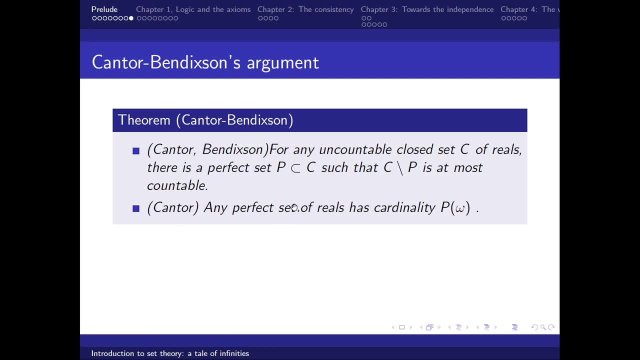 As then the analog of Cantor's mid-sert construction gives you that the perfect set of reals just have the same cardinality of the continuum. Okay, so that's just the Cantor reached when he was pondering his question about the size of the continuum. 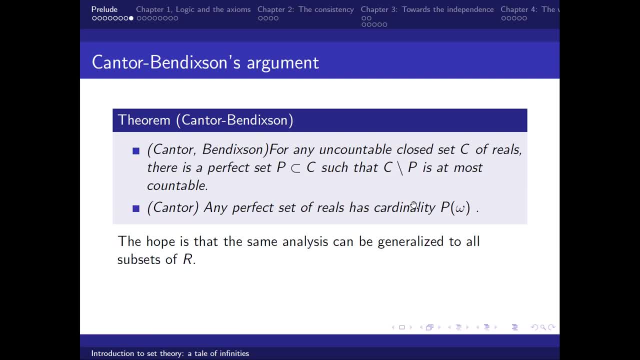 So his hope is that the same analysis can be generalized to all subsets R. Then we can just simply prove. it's not simple, but there is a proof for the continuum hypothesis. But the spoiler is that his hope is going to fall through. 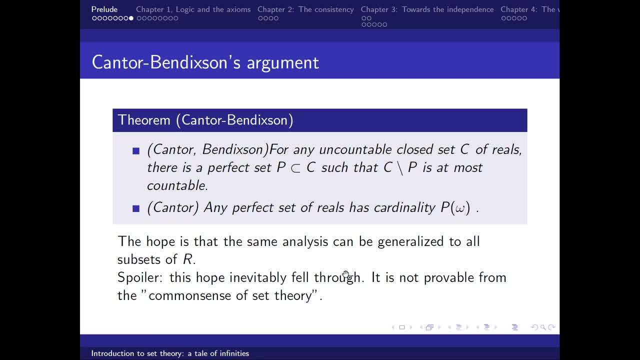 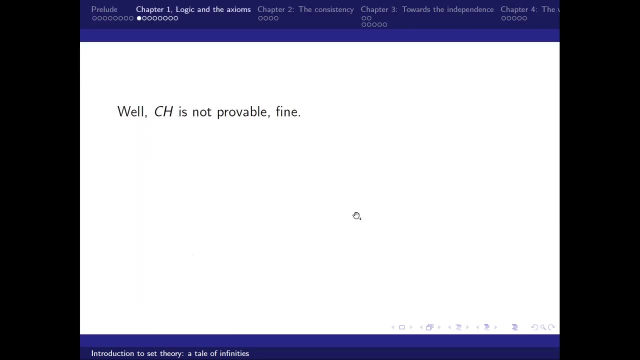 because it's not provable. I assure you within my presentation, how this is going to not provable. Okay, so the spoiler tell us it's not provable. Fine So, but wait a minute, what does that even mean? 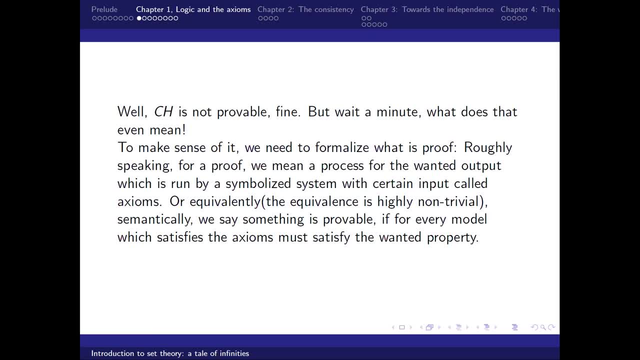 To make sense of it, we need to formalize What is a proof. So, roughly speaking, for proof we mean a process of a wanted output which is run by a symbol, symbolize the system which contains certain inputs called axioms or equivalently. I mean it can be listed in us. 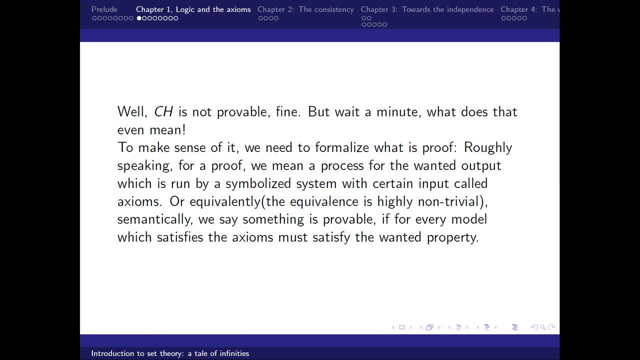 or it can be listed in a semantic way at the. they are shown to be shown by the other to be equivalent, but the proof is highly non-trivial. So another way to say that is that we just say that for every model which satisfies the axioms. 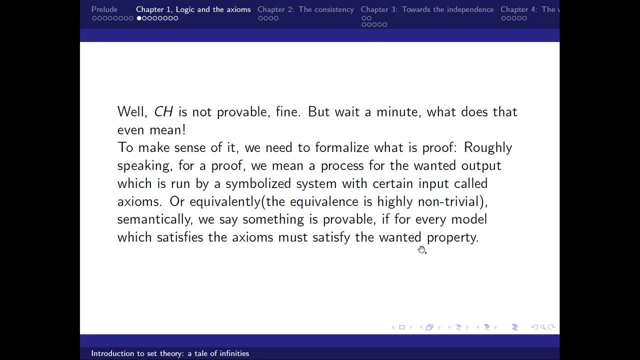 must satisfy the wanted property. But we need to formalize what proof is. I'm not going to do it here. I will assume that all of you know how to formalize the logic, concept, proof, the formulas, the sentences, So let's just assume everybody knows this. 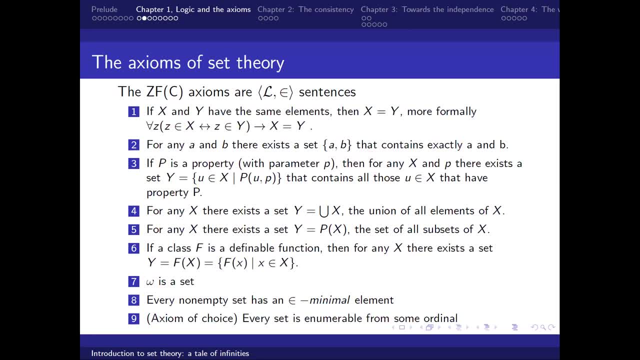 So I just going to show you the axioms of the set theory, of set theory. Okay, so there are a lot of axioms, but I'm going to explain. what does it mean? So the first one is called the axiom of extensionality. 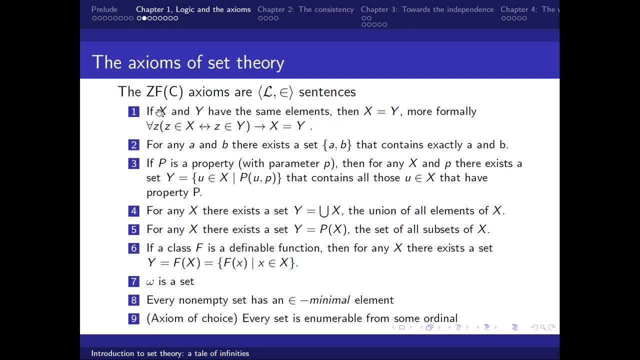 which says that, okay, no matter what the names for the set is, whenever they have the same member they are the same thing. So we can formalize this sentence into the by our L epsilon language. So that says: for all the if they is in X. 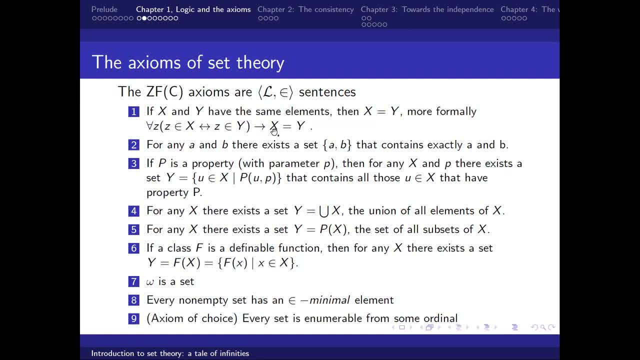 if only. if they is in Y, then X is the same as Y. So okay, that's reasonable, right? Also, that's our intuition about sets. So the second one is that if A and B are set, then we can just collect them. 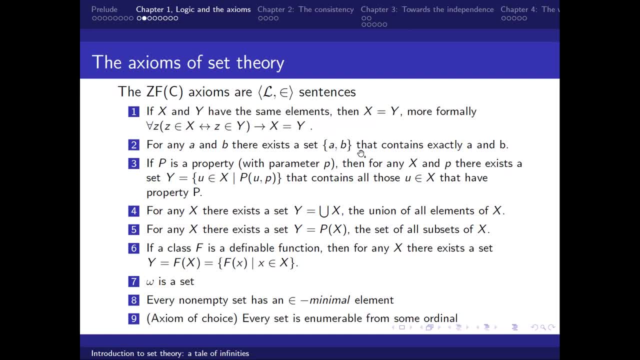 That will be a set. No one will disagree with it. right? You have two objects, Then you can have a. there is a set which contains exactly these two elements. Okay, Third one is the power of set theory, which essentially says that whenever a piece of object 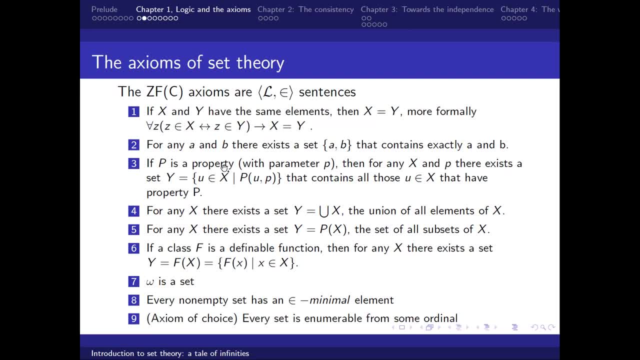 is in the set is a set. So that is a set is a property which is described by some formula in our L epsilon language. So for any set X at a parameter P, the subset of X which is decreed by the property P, 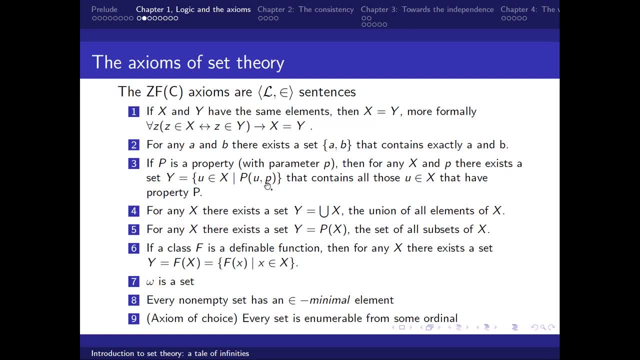 with parameter P. for some P, I mean, if you don't have that parameter, it's also fine. So such a collection of elements in X must be accept into our set theoretic universe and it is a subset of H. So Y is in. if y is just a collection of elements of X, 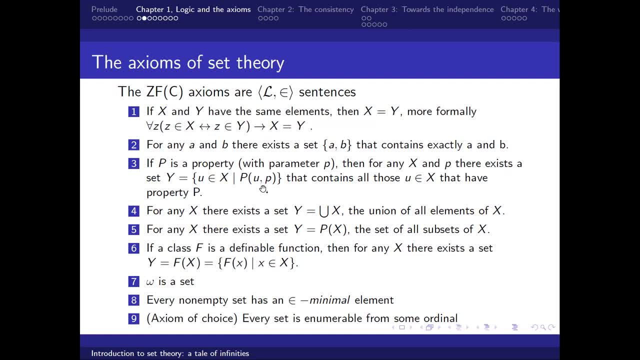 with certain properties. That's fine, right. For instance, if you have the set of all nature numbers, you accept that the set of nature numbers is in. So the set of or the set of all even numbers is just the subsets defined in this way. 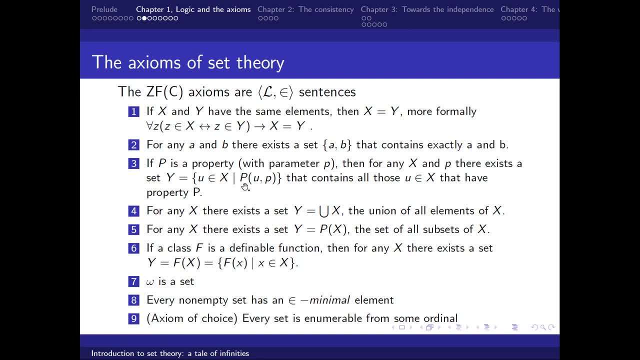 So there exists the Y, Y plus Y is Z for Z in X. So that defines the set of even numbers. So okay, that's also reasonable. So the first one is just says we can take unions, So I mean so for every X. 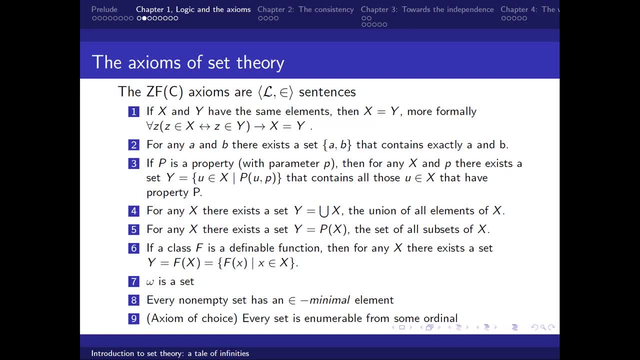 so X is a set of sets, So Y is the union of the elements in X. That's going to be a set. It's also reasonable, right As the fifth one is that if X is the set, then the set the collection of all subset of X. 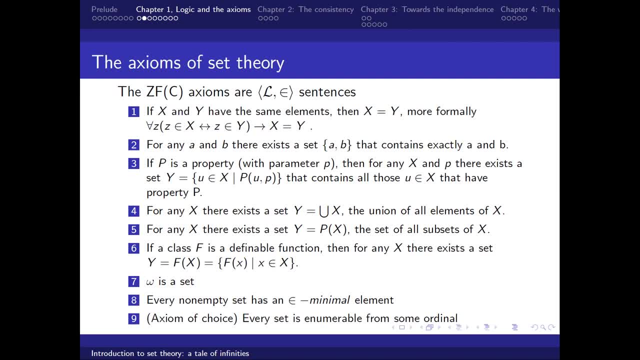 must be a set. Well, that's how we perceive the. I mean, the set should be right: You have a set, so you just collect all of its subsets. Is it going to be a set? Yeah, I think so. 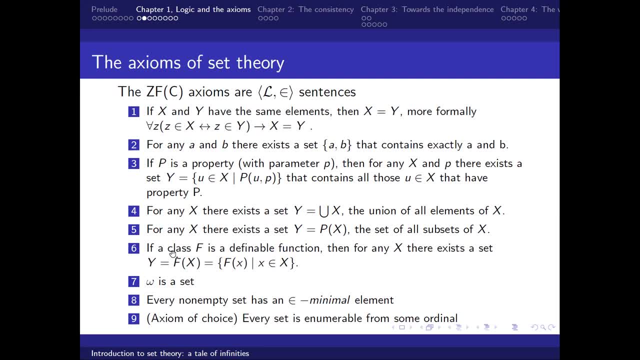 At the sixth one is the axiom of replacement. So what do you mean by replacements? So let's suppose phi if it's a definable function, Equivalently if it's defined by some formula, again in our L epsilon language. 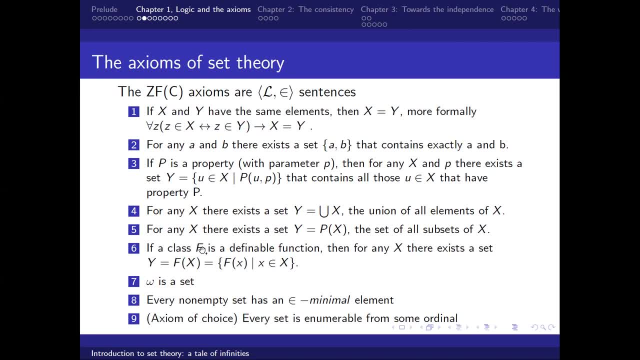 But it guarantees that for every input there is just there is only output. So that is what I mean. So that's the definition of a definable function. So okay, So this axiom says: if X is a set, then its replacement by such an A must be a set. 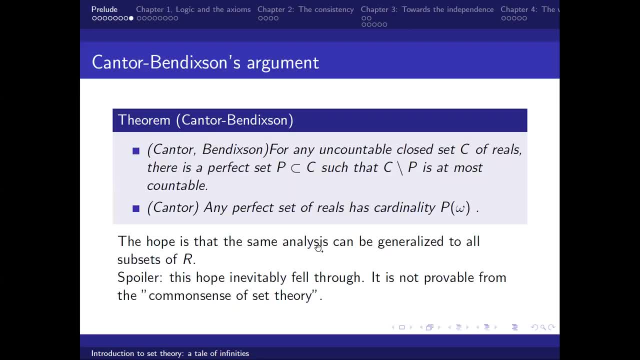 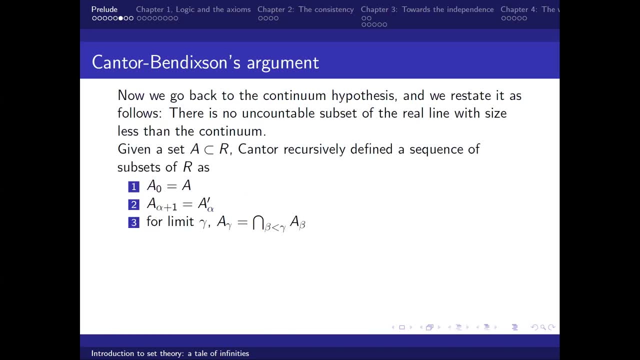 Okay, let's just go back to the, to some statements that I promised to give you some explanation of, So let me go through after I went through the axioms. So here: so Y is a set. it's going to be a eventually constant. 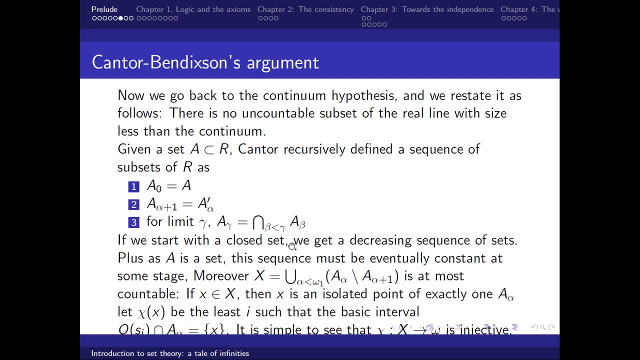 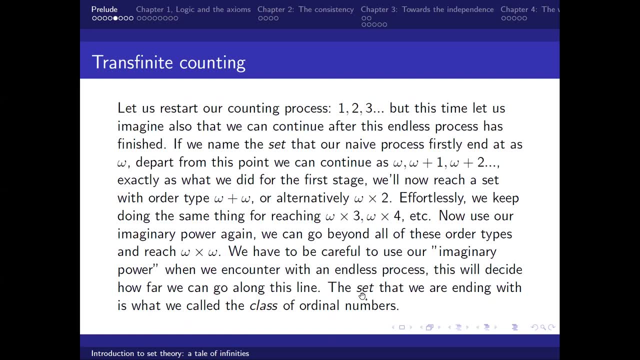 because if it's not, it's going to be mapped somehow to the universe of the ordinal numbers, right, By replacement. we can replace it to the class of the set. So it's a class of all ordinal numbers, But again it's our universe. 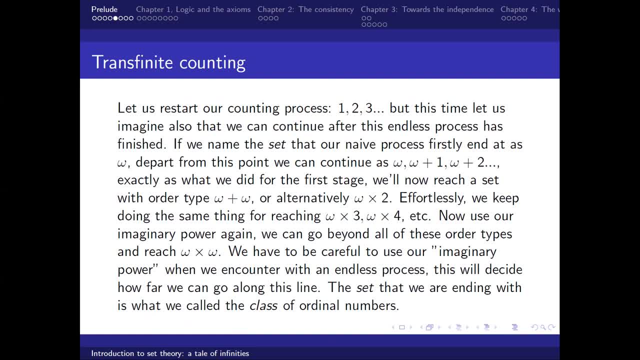 So we cannot, you know, go over it. It's just where we are going to end, Since if we have a set of all ordinal numbers, then we are going to carry out the same process after it. So it's not going to be the set of all ordinal numbers. 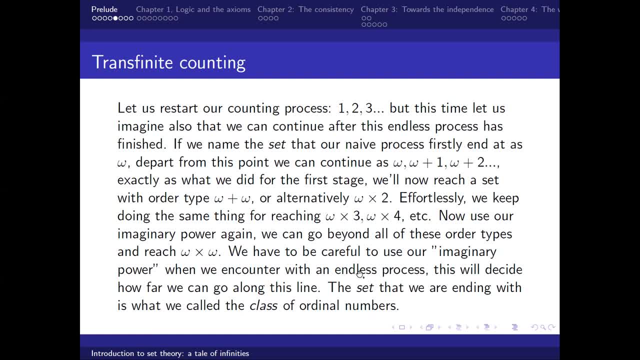 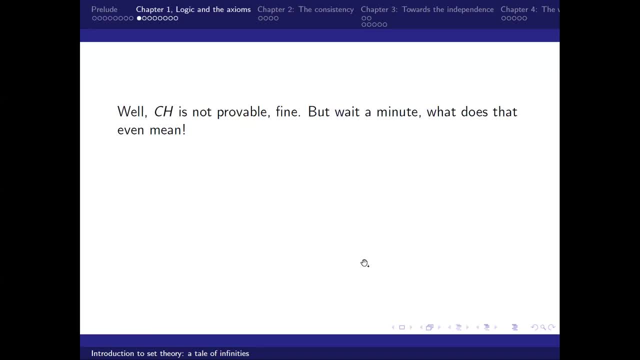 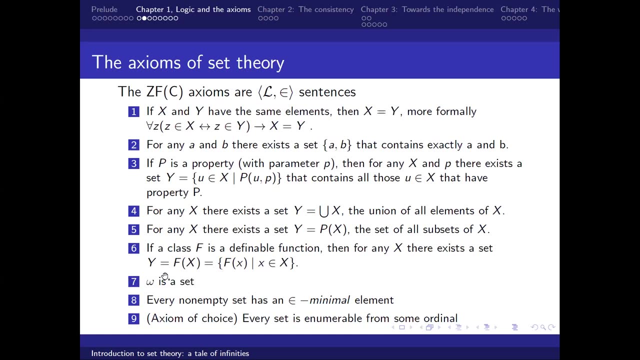 So it's not going to be the set of all ordinal numbers. It's going to be the set of all ordinal numbers, Right, Okay? Then there's a first large cardinal axiom. So we assume there is a event set and also we assume that universes we'll find. 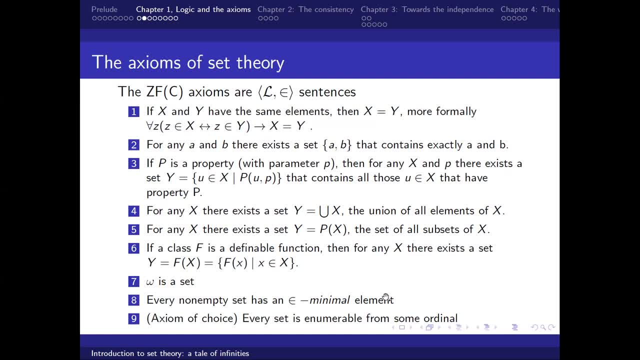 namely it has a set e, and also we assume that universes we'll find has a solid foundation in terms of sets. I will explain. seventh eighth condition later on. At last one is the axiom of choice. I mean, it's an equivalent way to say that. 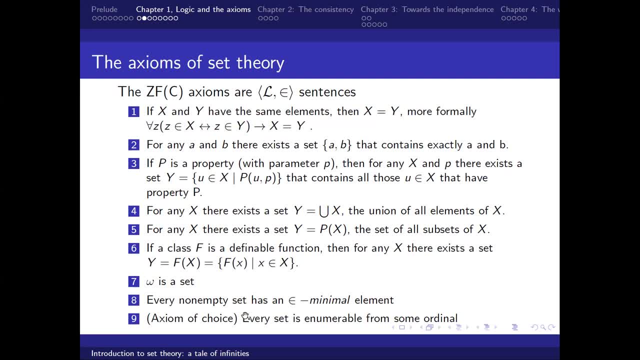 but I'd like to present it this way because we are counting numbers. So this is actually the strongest way to state the axiom of choice, regardless of the rest of the theorems. So it says that every set is actually reorderable, or say every set is enumerable from some ordinal 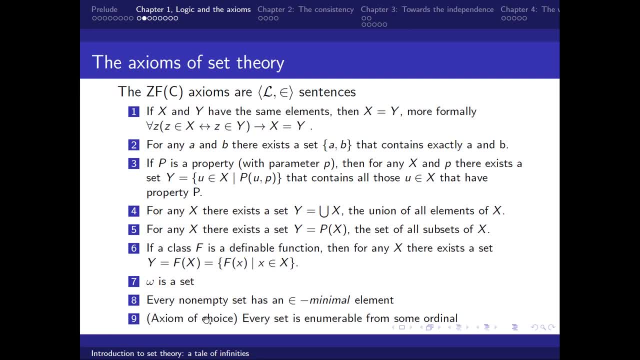 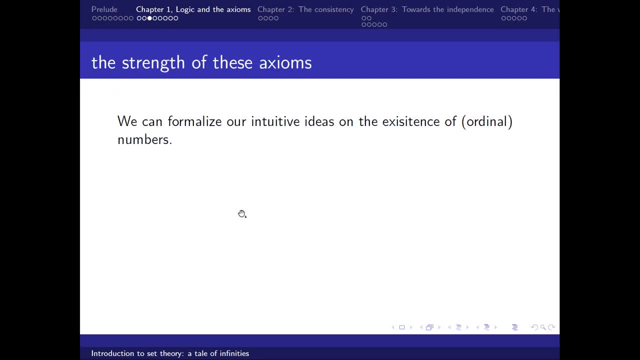 But I'm not going to go into any details of axiom of choice, I'll just leave it to my colleague. Okay, So with this axioms we can just reformulate the ordinal. We want to show that ordinal actually exists. So historically this was firstly done by Cantor, of course. 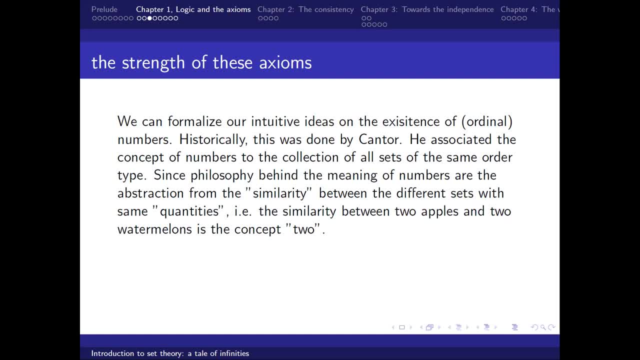 So the philosophy behind the numbers is general, just the way it extracts the similarity between two different sets with same numbers. Imagine that. so what's the similarity between two apples and two watermelons? So it's a concept too Okay, but you know how can you present the? 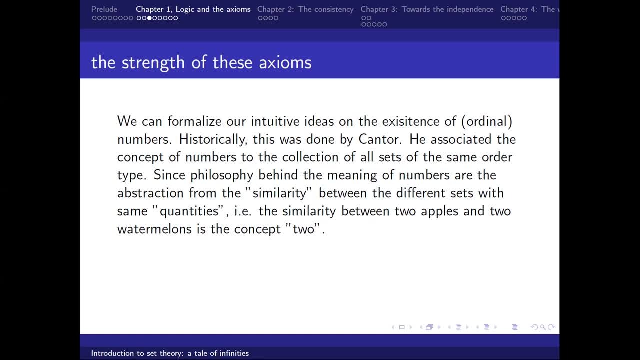 represent the number two out of that. So our axiom: just grant us powers to do that. We just collect all the sets of the same order type to represent that order type, And it's a set which we can, you know, use as a representative for the order type. 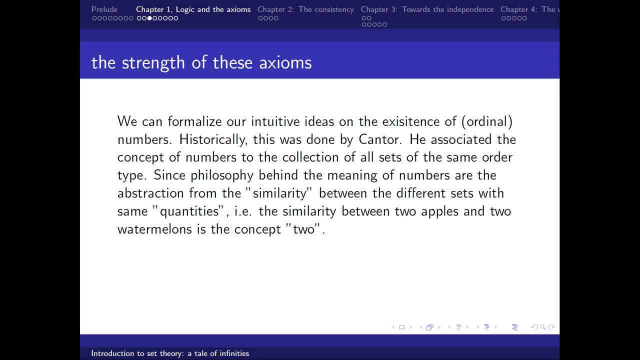 So this is a standard way of how set series work. So you can see by the virtue of the axioms. let's say how to characterize two in the original way by a candle. it's just the collection of all sets, which consists of exactly two numbers. 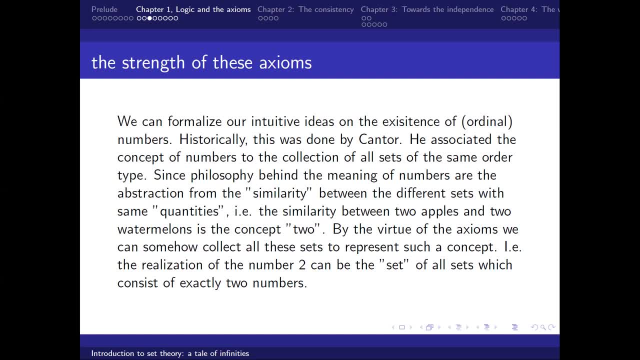 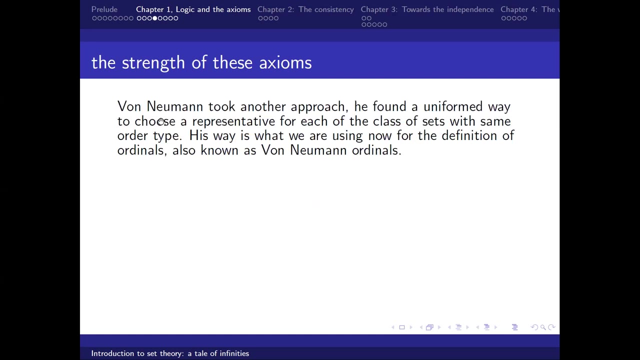 Okay, so that's the whole thing, but it doesn't give the order or any more information about the ordinals themselves. In fact, we have a better definition later on by Von Neumann. so Von Neumann took another approach. He found a uniform way to choose a representative. 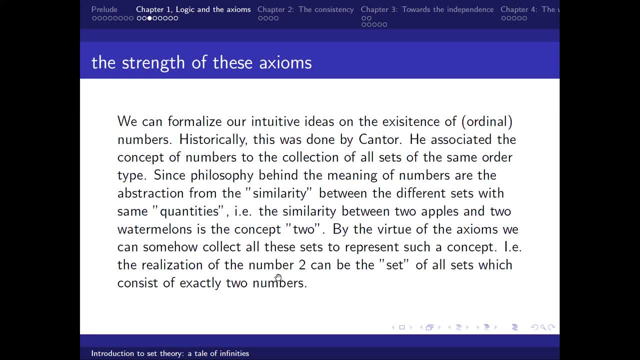 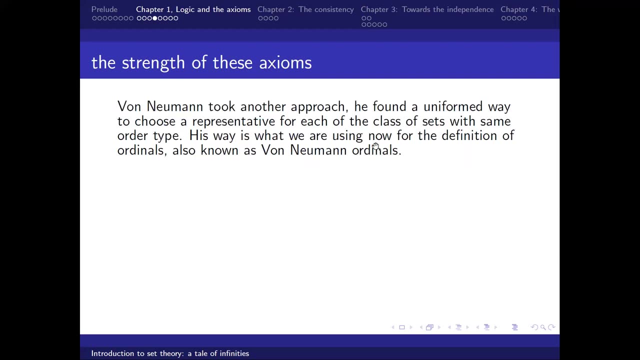 of each of the class of sets, namely for two. yes, He choose a member of the collection of all sets- exactly two members- as the representative for the number two. So his way is still in using because it's very good, I mean the set itself. also have a lot of information. 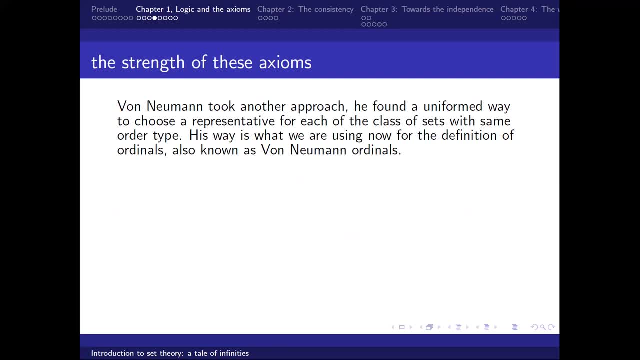 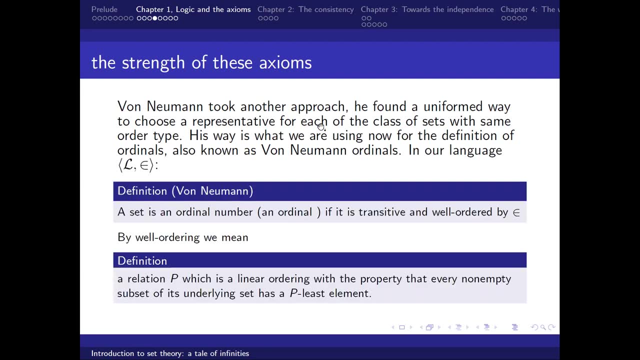 So that's very convenient for using. So there's ordinals known as Von Neumann ordinals. So again we have to work with our language, L epsilon. So this is definition given by Von Neumann. So a set is an ordinal number or an ordinal. 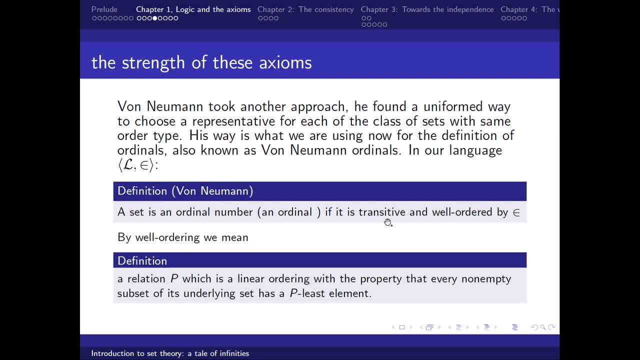 If it's a tracitive set, namely for every X which is a member of the set itself, it must be a member of the set Plus. the membership relation is a real order relation of such a set. So by reordering we mean a relation P. 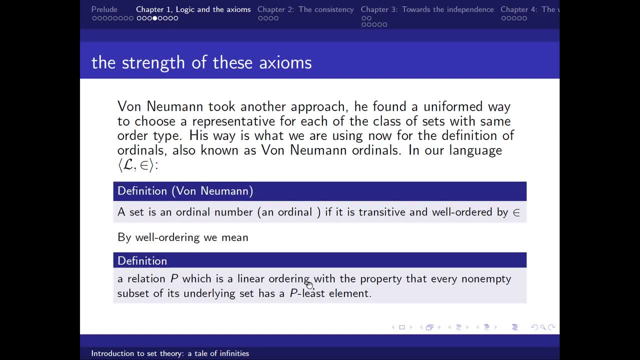 which is a linear order, namely it has a trichotomy. It's a trichotomy Tracitive, So false. Where is the property that, for every non-empty subsets, it's underlying set has a of its underlying sets? 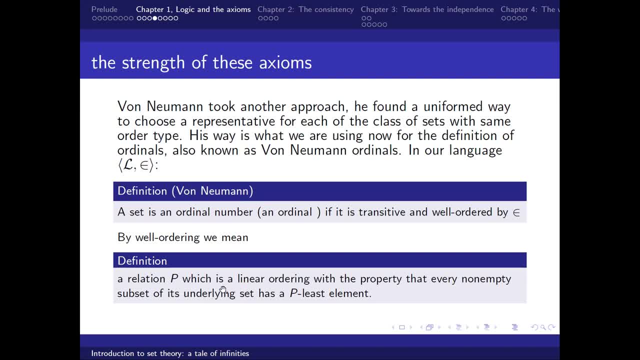 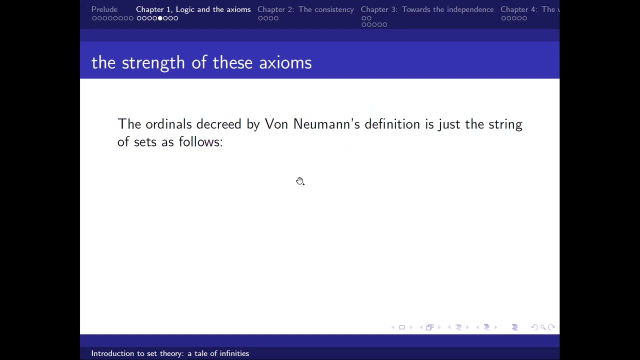 So the relation has underlying sets, So the adding subset of that set has a P least element. Okay, So let's move away from the abstract definition. It's actually a very concrete thing that we can work on with, So let's just try to see why this works. 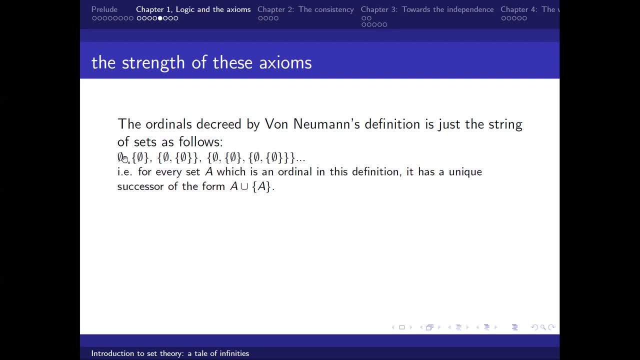 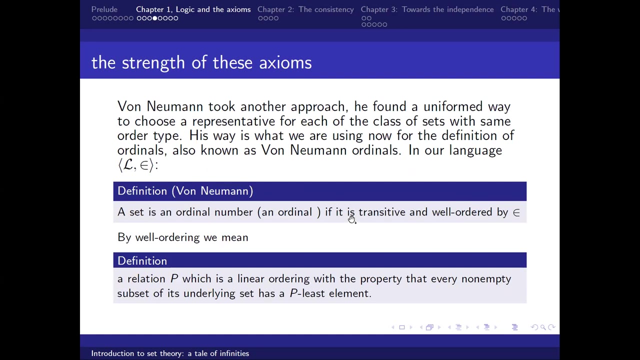 So first, the first one by foundation, by the axiom of foundation, must be the empty set. So the empty sets will satisfy the criteria. First of all, empty set is tracitive because it doesn't have any member of it. So this is a we can actually true. 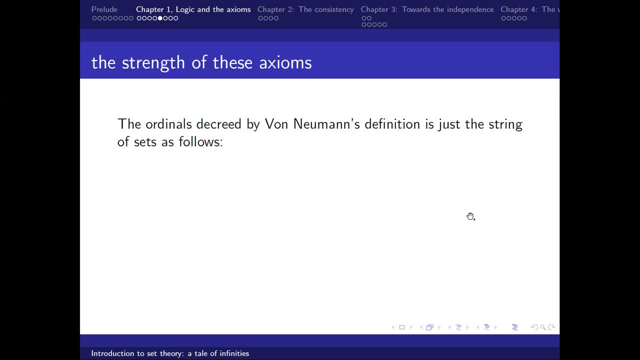 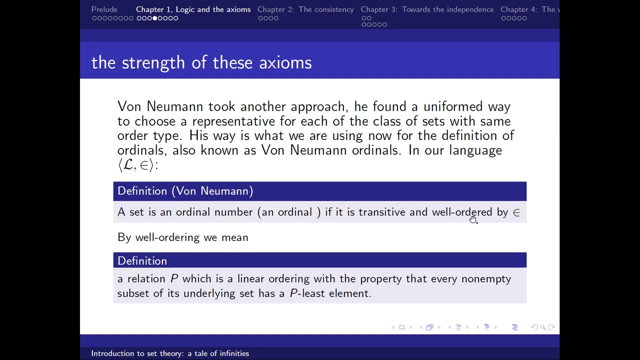 And also this is true, And for this one sure only have one element And there's no elements of the element of that set. So the first one is true. The second one also is weakens to be true because there's only one element. 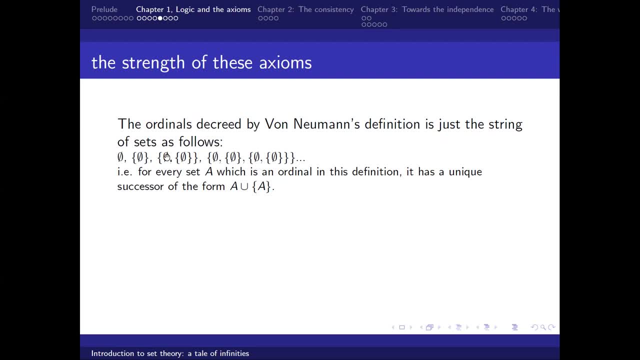 And the third one you can say the element of empty sets is we don't have any, So the tracitivity with respect to the empty sets as a member of this whole set is not going to ask us to add any members into that set. 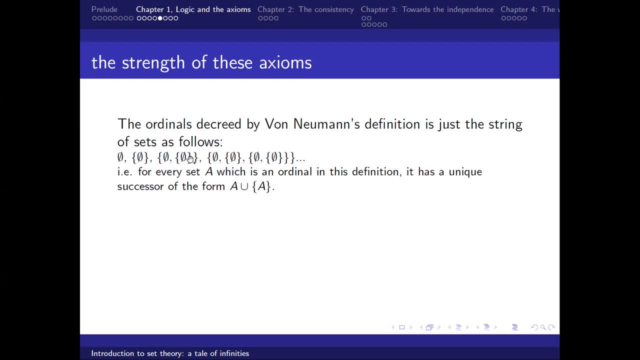 How about this set? So the tracitivity means that the members, the member of that set- is a member of the set. Okay, So this is the whole set. Okay, What's the member is? the member is empty set, but it's already in. 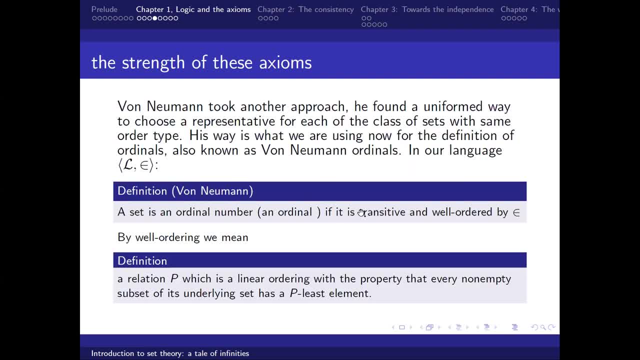 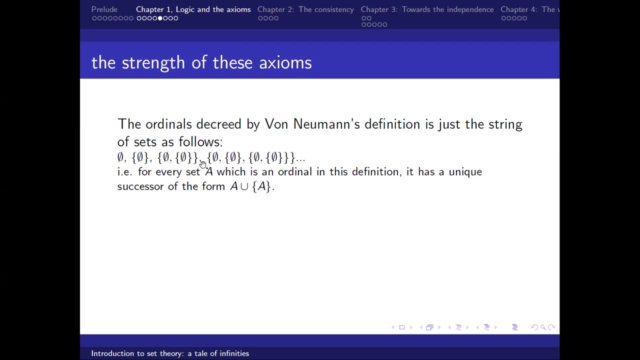 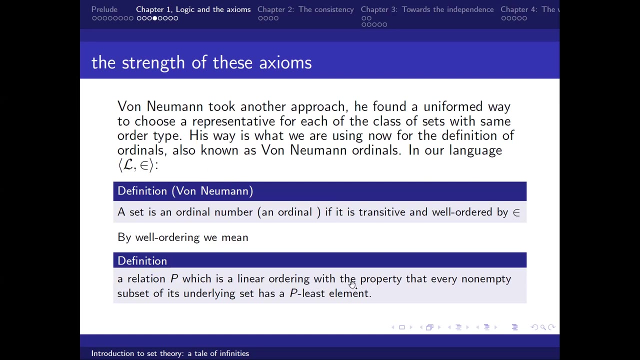 Okay. So tracitivity, Okay. So the third one is tracitivity. How about the way ordering by the membership relation? Is it a partial order? Yes. Is it a way order? Yes, Okay, So adding non-empty subsets of this set. 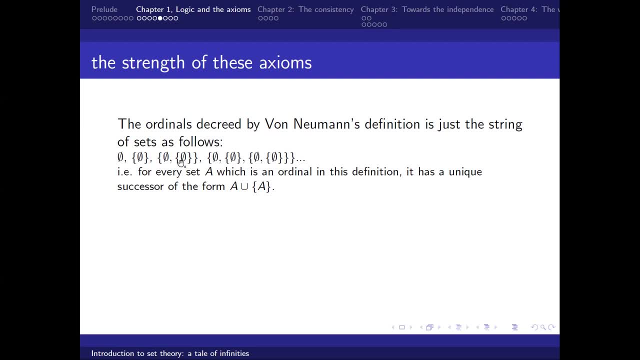 has the least element under the membership relation. I think so. If it's a whole set, it's an empty set. If it contains empty set, it's going to be empty set. If it only contains the second component, it's just going to be it. 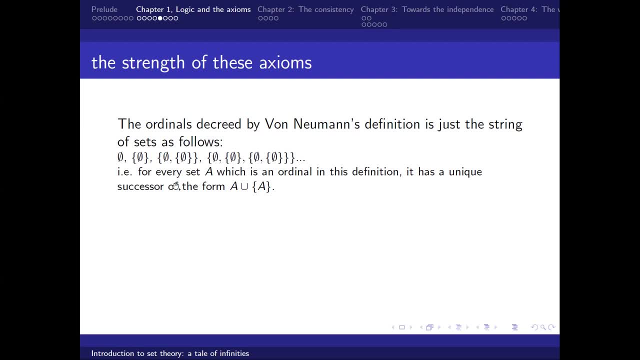 Okay, So false, We can carry on going. So how I construct this set? Yes, So it's just the tracitivity inductive construction. Start from the empty set. You keep adding successor to it. So whenever you have an ordinal 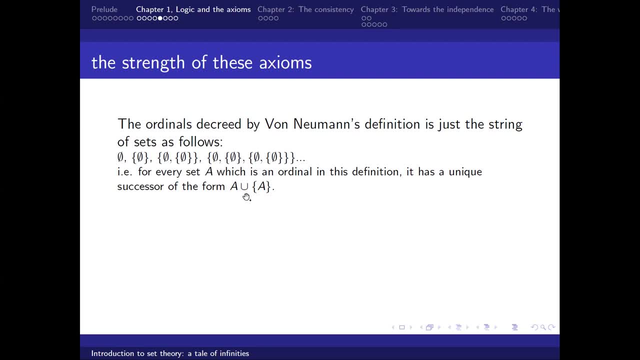 it has an empty set. Okay, It has a unique successor which just takes the ordinal and union it with the singleton of itself. So this is how I construct this whole thing And you can see from the very construction of this ordinal itself is very informative. 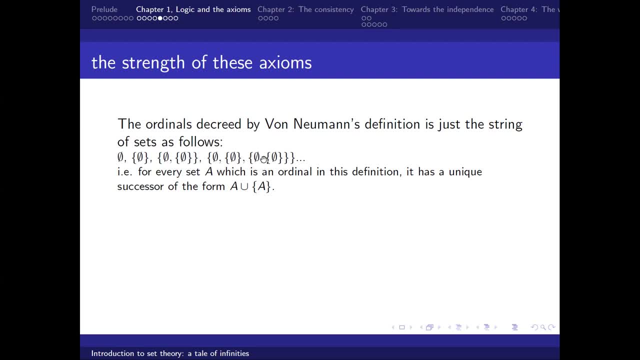 because you can see, the membership relation just gave you the way of ordering. I mean, so the way of ordering of that set is intrinsic. I mean that's one of the merit of this definition, But overall it's a very nice way to define it. 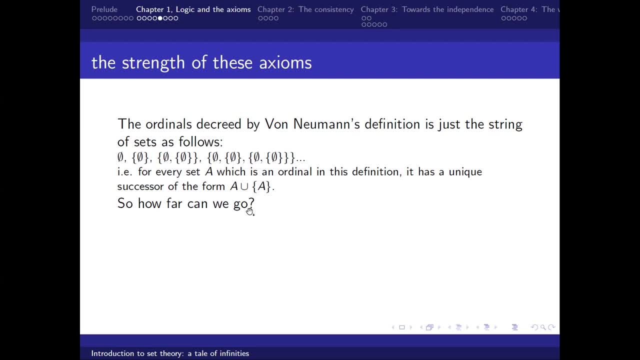 Okay, So move away from this Again, back to the slides. that, how far can we go? Okay, So now we have our axioms. I'm going to show you that the first uncountable ordinal must exist as a set. 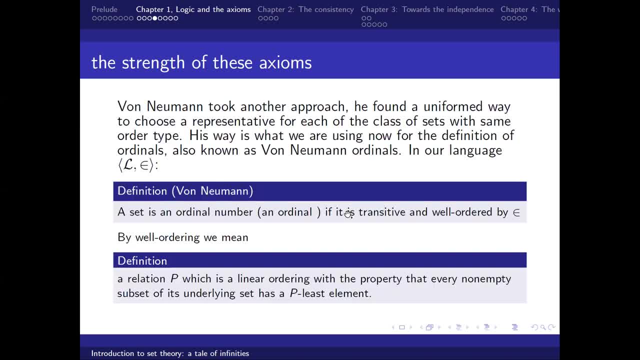 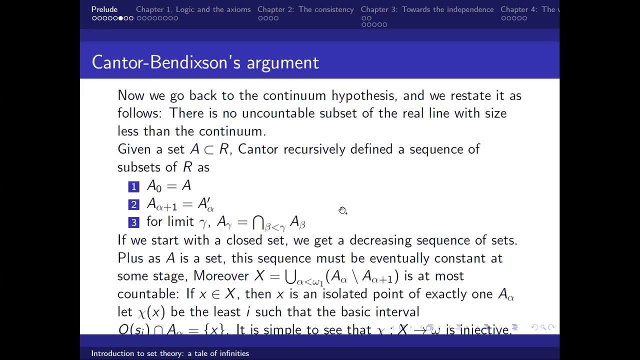 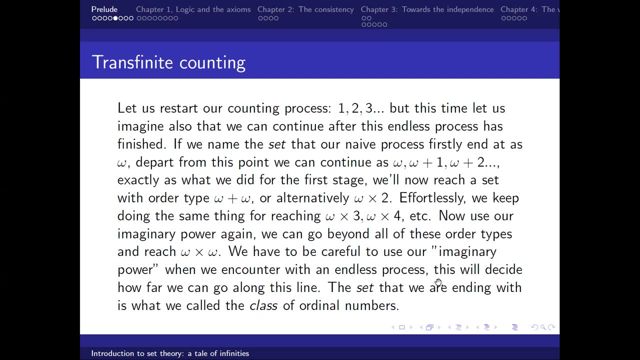 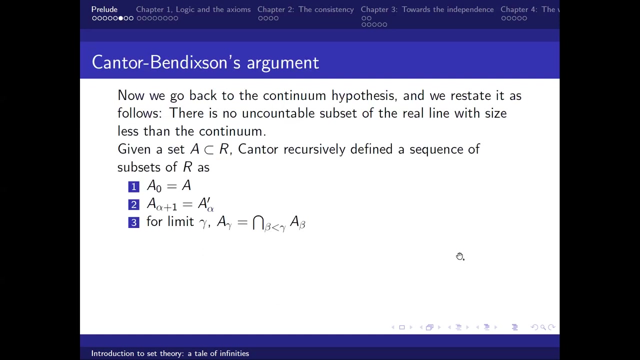 Namely the ordinal, the ordinal line roommates. so the ordinal line is not just the collection of countable sets, So we can pass us through the countable universe where the whole thing as just the element of our universe. So 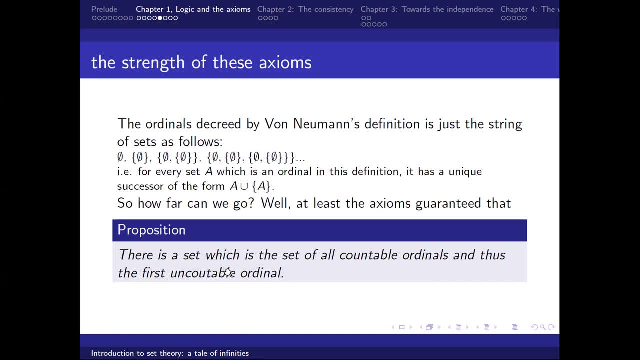 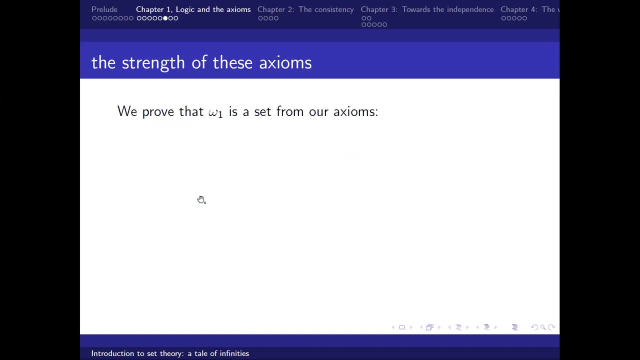 the first uncountable ordinal where we call omega1, it's not going to stop us. So we prove that omega1 is a set from our axioms. So for that we need some preparation, Do some codings or somethings within our framework. So let's say, the first preparation is that for 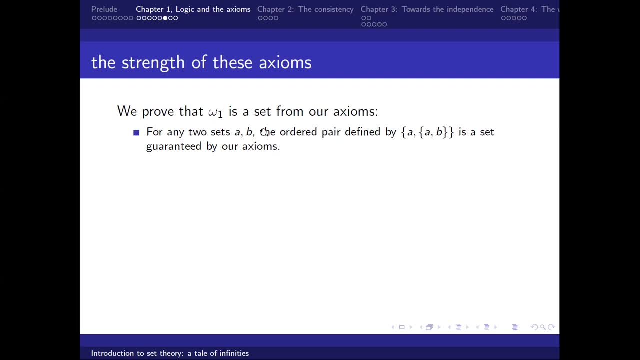 adding two sets, a and b, we can construct a set which is called ordered pair. This represents there is a pair which consists of at b, but we can tell the order between them. so which is the first component, which is the second component. so there is a way to represent an ordered pair of a and b. so this is a set guaranteed. 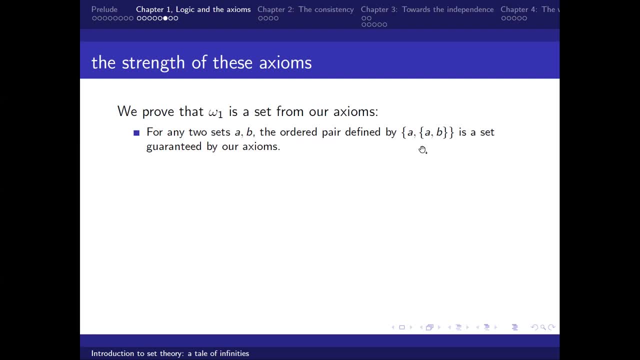 by use our, if i remembered it correctly, by our second axiom twice. okay, we have ordered pairs, so we can use the collection of ordered pairs to formalize the relation on a given set. so, whenever we have some relation on a, how we translate it into the very construction of the sets which can 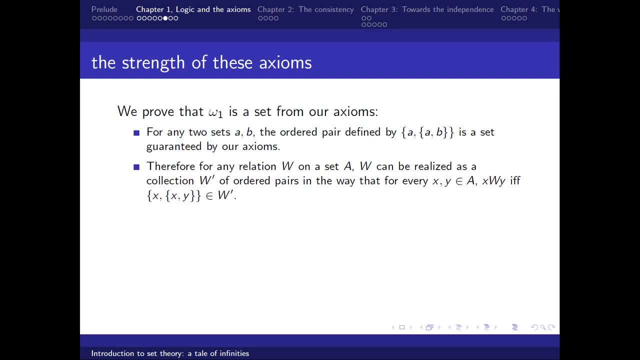 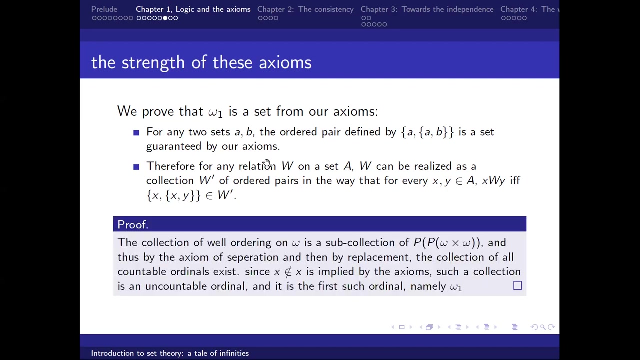 represent the relation. well, it's just a collection of the um, of the ordered pairs. so which shares this property? so if x is z has w relation with y, if the ordered pair x and y is w prime, okay. so, after the tedious preparation, i can show you why omerta y exist. 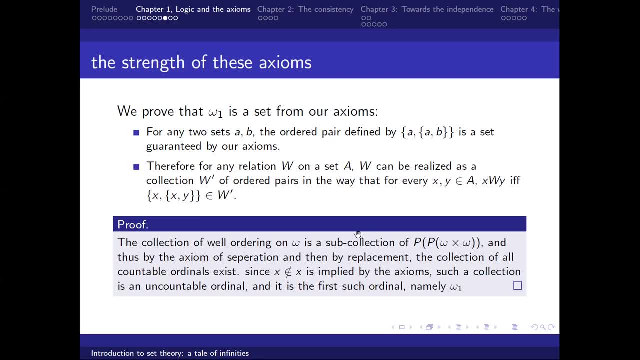 so essentially, you can just take the collection of all of the ordered pairs, all countable. we're ordering for omega, So are we ordering an omega? It's just a relation of omega If we code this relation in this way. so okay, the collection is then. 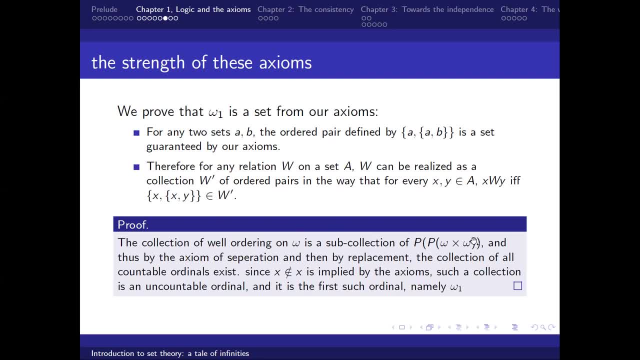 just a member of this set. Then again, by the axiom of separation, we can separate the well-ordered well-ordering out of all subset of subset of omega, cross omega. So it must be a set, So by this definition, the set of all countable well-ordering of this set. 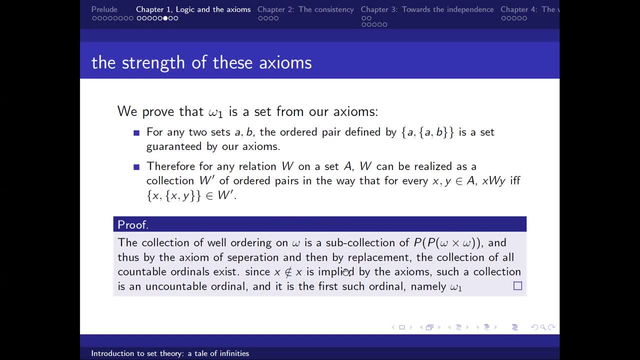 can be replaced. It can be replaced by the collection of countable ordinals along the von Neumann line, As thus it's going to be an ordinal, of course, but it also has to be uncountable, because if the collection of all countable ordinal 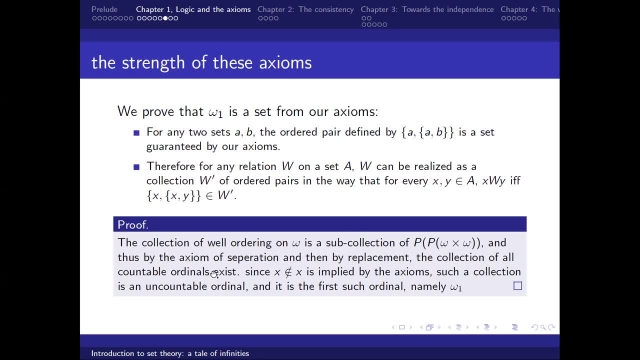 is again a countable ordinal, then it must be yin itself, which is not possible by a lot of the axioms, For instance our axiom of foundation. So the collection must be an uncountable ordinal and it also must be the first such ordinal. 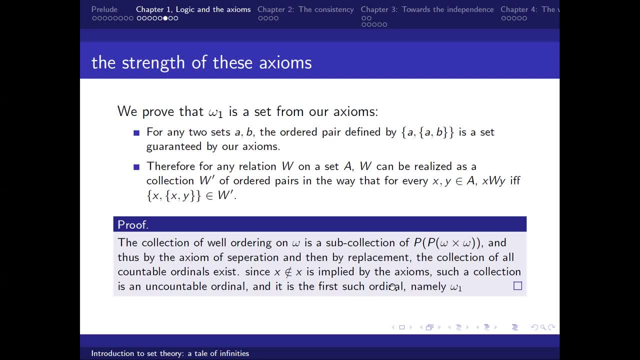 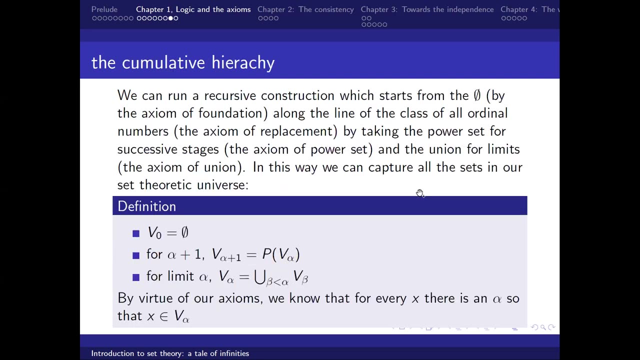 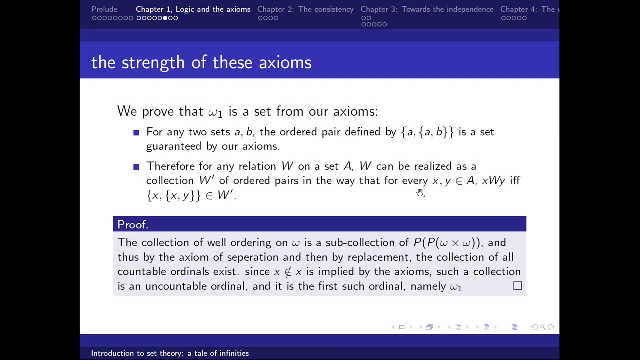 because any elements of it is countable. So it's the first uncountable ordinal. we call that omega y. Okay, So that's, that's the first observation about our ordinal line. So work with that ordinal line and then we'll get to the next step. 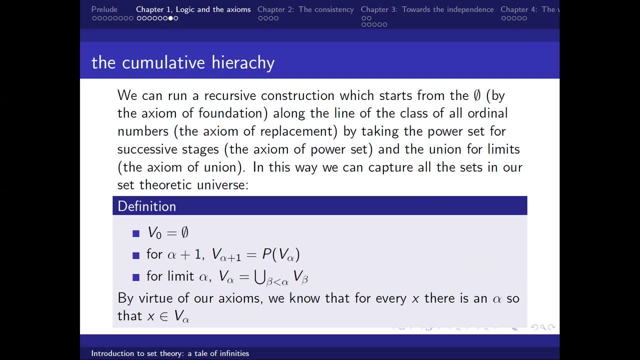 We can essentially use the parse set operation as the union operation to capture all of the sets in our set theoretic universe in the following way: So we start with the empty set. At successor stage we take the parse set of them. 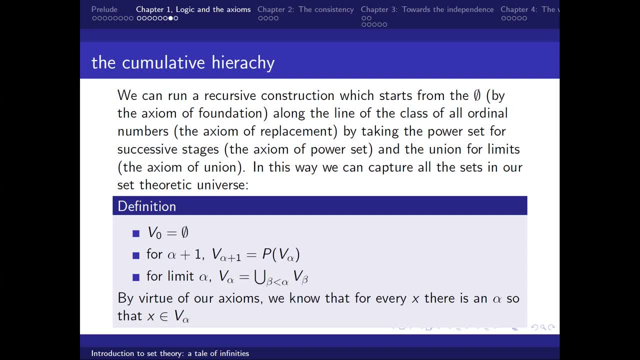 and we do an order search, set At the for limit stages. we just take the union of all sets, all hierarchies that we have already got Okay by the virtue of our axioms. all of this, I think especially. 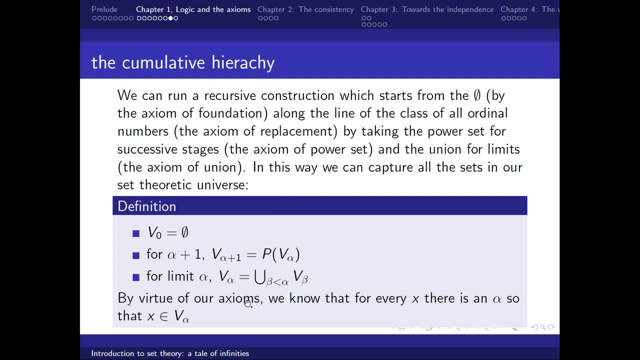 for the axiom of foundation. we can actually prove that for all x there exists an alpha and that x is in the alpha. Okay, this hierarchy is called the cumulative hierarchy. Okay, I will just Okay. I will just Okay, I will just. 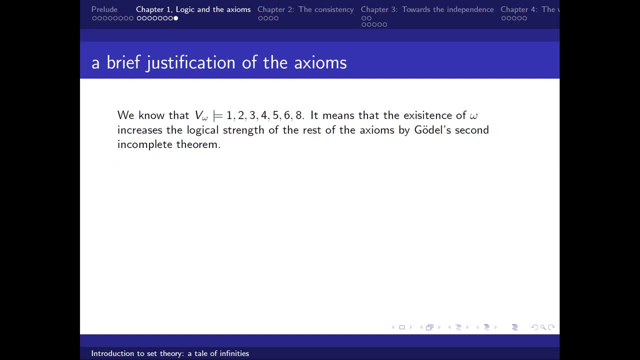 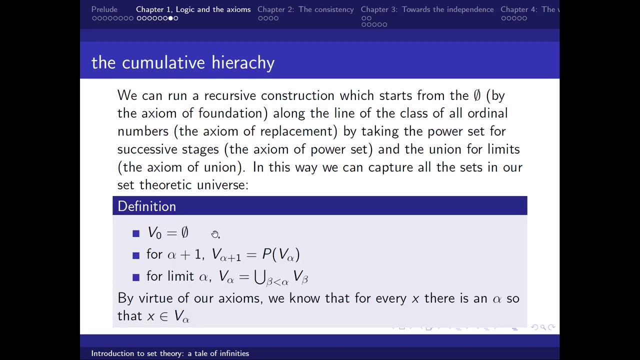 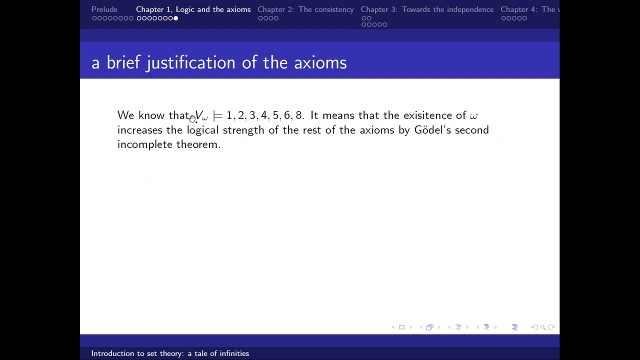 give you a brief justification of this. axioms again. So if you look at our cumulative hierarchy, let's just stop at the stage omega. So, let's just stop at the stage omega. So if you look at our cumulative hierarchy, let's. 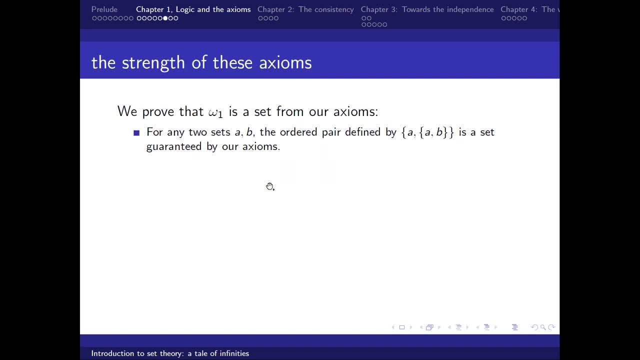 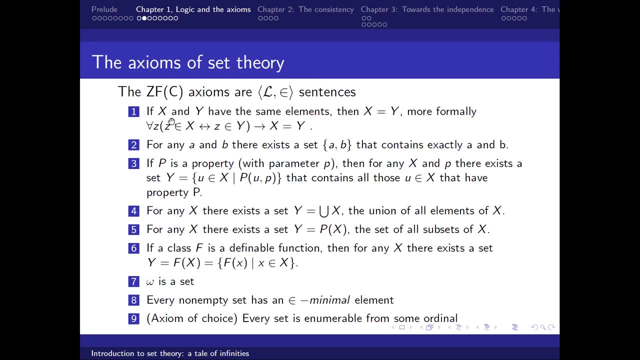 just stop at the stage omega So we can see that the the we learned from weight omega. We know that the weight omega satisfies a lot of axioms, So of course it satisfies the first one and the sixth one. no problem, because when you are taking, power sets you. 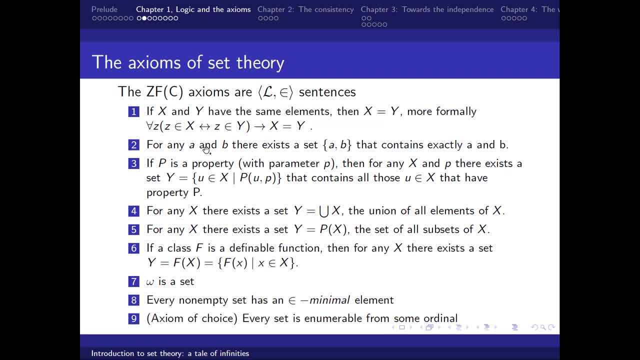 just add all of the, the omega's in the data And if you um, all of the, the subsets in um the third one, of course, no problem. i mean, we just assume that we, we, we've already worked in some sincerity universe which satisfies the. we are, we are looking at. 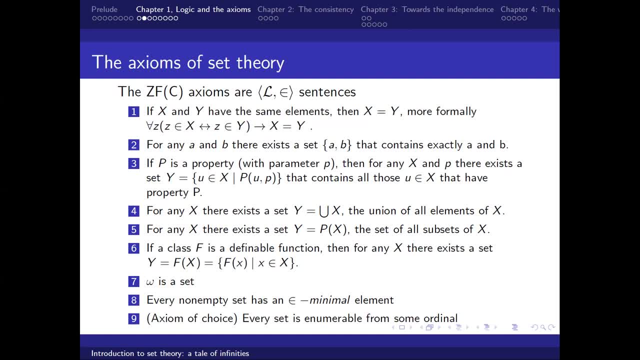 with omega, of that, of that model. so the third one: yes, sure, i mean because that's a initial segment, where omega is the initial segment, or they have, they have the models, then union, no problem. yes, power sets, that's what, what we do, that's replacement. okay, because we are stuck in with omega. so i mean all the x's. 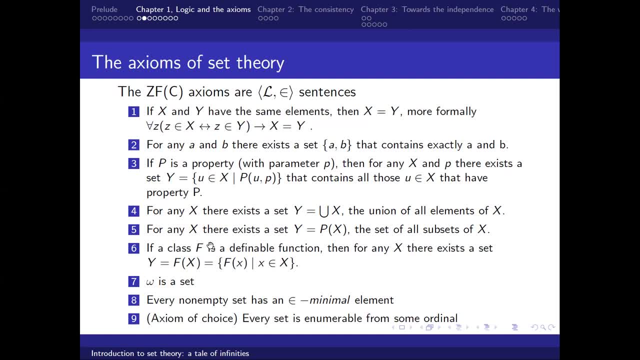 must be a finite function. but f is a definable function. that means for every element it has only one image. so y is again must be a finite set. it's him, no problem. how about the a-spline? yes, sure, no problem. nine is also preserved, okay. 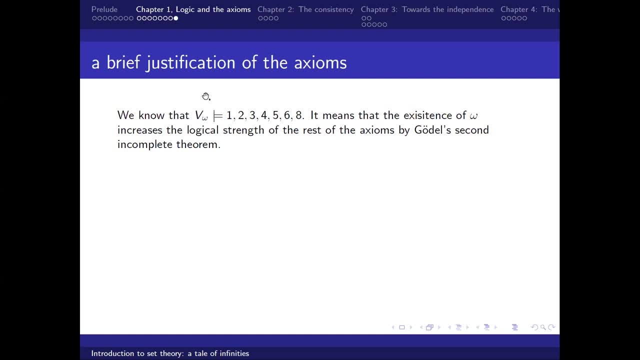 so if we have a way as a model of our zfc, and then if we have a way of omega, and then if we have a way of the x's, and then if we have a way of omega, and then if we have a way of the axioms, 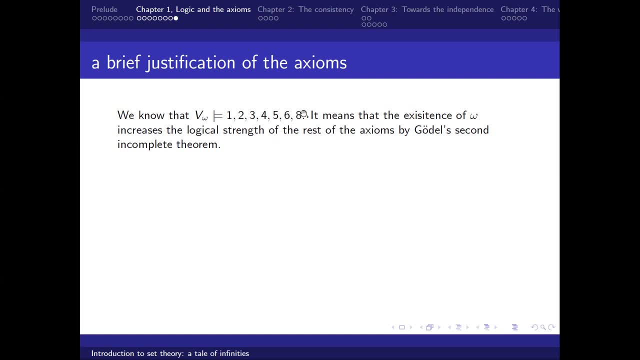 then its way. omega is just the model of all but the axiom of infinity, so that would mean that the existence of omega is actually increases the because the rest of the axioms can actually prove, I mean, can interpret the piano arithmetic, piano arithmetics. 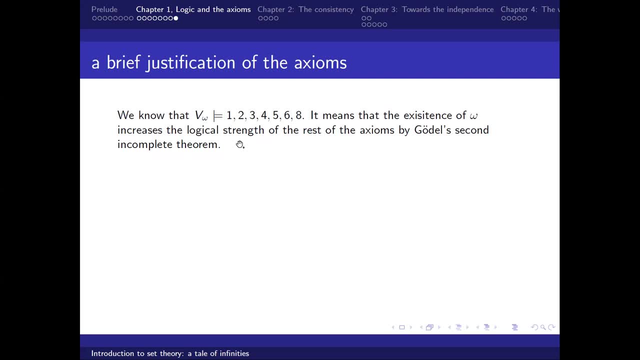 than the Goddard's second completeness for a suit. So namely, they cannot prove so from one to eight, but seven cannot prove the consistency of itself, but with the seventh you can. So why we? I mean all of this. 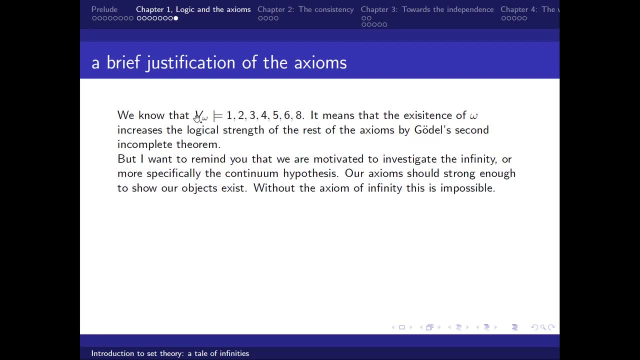 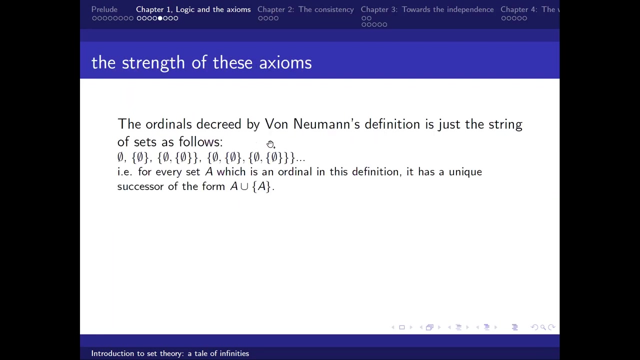 all but the seventh one that we just demand. there is one: the infinitary object being is. I mean, it's obvious if we, we are even working within the finitary universe, right? So if everything is finite, if everything is finite, 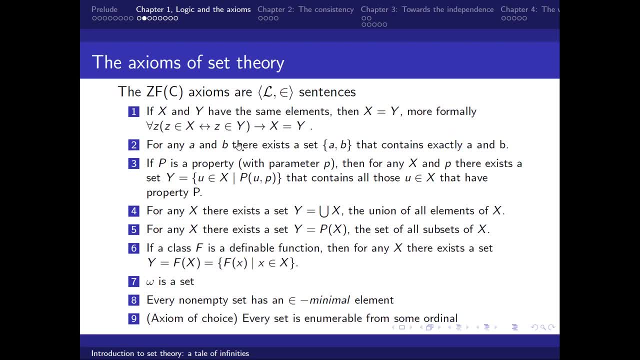 so one is true, right. Two, why not Three, for a finite set. okay, the we have a property. Okay, we exempt. we exempt one by one. So which one? So for each element of the given set, X. 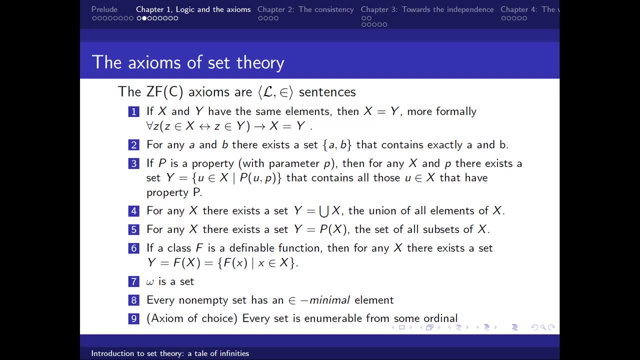 we just ask if the property holds for that element or not. Holds in doesn't hold out. okay, that's a very intuitive way to form a set. Why? I don't see why that set Y shouldn't be in. You take the union of the sets. 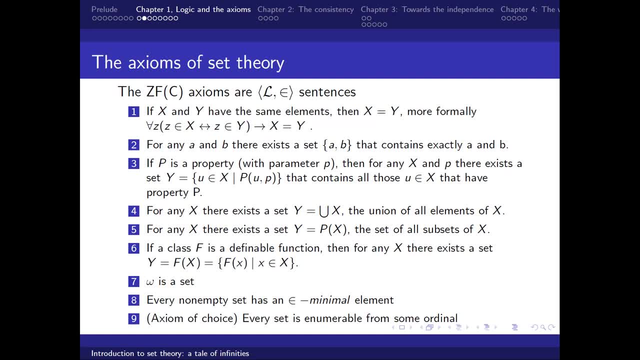 Let's say we have a finite collection of sets, So each one have some members. We just take the union of the finite sets. fine, Why, I mean still, obviously it should be in the power set of it, Of course. 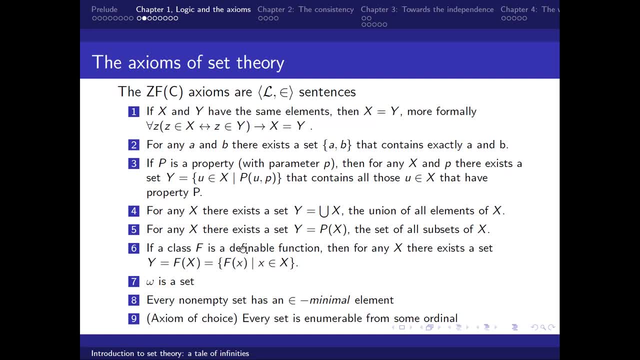 The replacement, of course, the foundation. Okay, start from the empty sets, Just go through the finitary stages. It satisfies this, Why not? The axiom of choices is vacantly true, because for any finite sets we can pick without any problem. 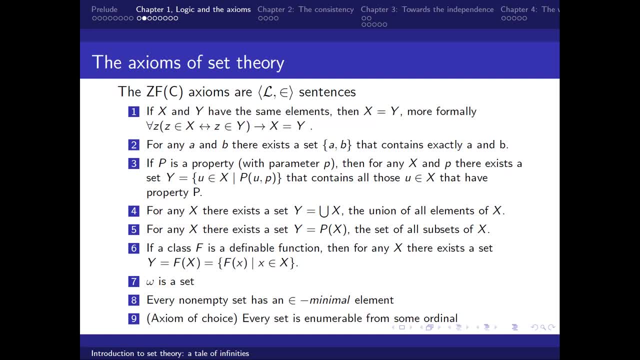 For any sets. we don't have choice problem. We just pick something out of it. For two sets, we just first pick one element of the first set, then the second, the one element from the second set, no problem. So if we stay finite, everything's okay. 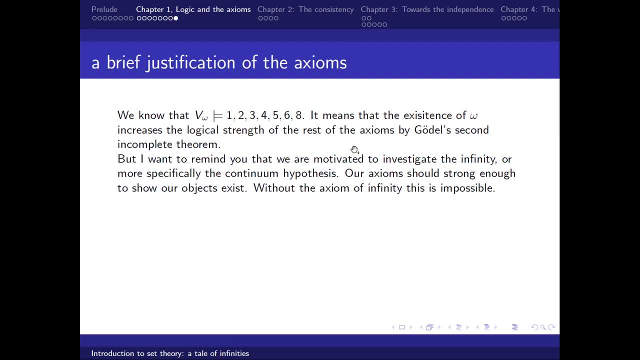 But if we add one more thing, this whole thing is going to be more sophisticated. So why we want to make this whole thing more sophisticated? Because at least we are motivated to investigate the continuum hypothesis. At least we need to have that. 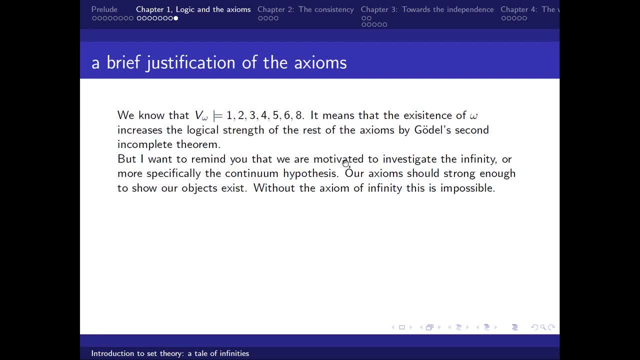 At least we need to have that, at least we need to have that proposition, to have that set in, but without adding the infinite objects outright. the rest of the axioms doesn't apply to this one, So we have to add it in. 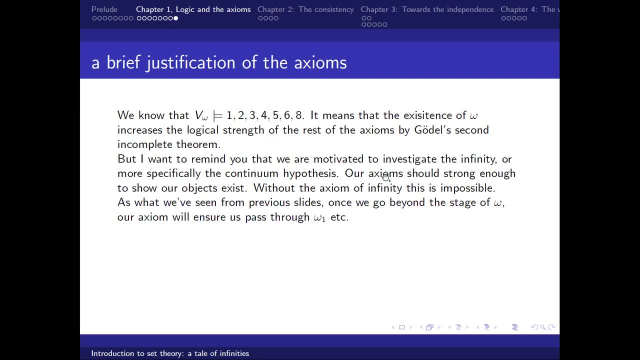 Add a is what we've said. It's going to be fruitful because once we add it in, it's going to give you a very rich universe. You can imagine that omega y is in, omega 2 is in, so forth. Suddenly it's going to grow quite big. 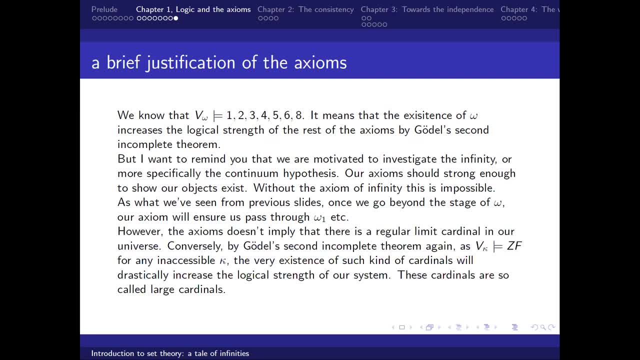 How big is this? Okay, well, there is a finish line. So unfortunately- or someone views it, fortunately- the axiom doesn't imply a regular limit, cardinal in the universe. So the regular means that it has the same commonality of its size. 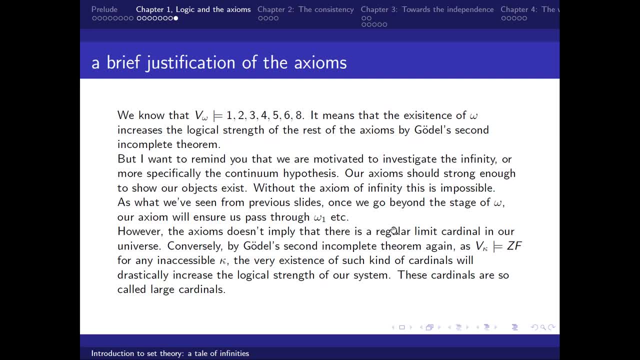 So a commonality function is just a co-final function in the sense of the membership relation. So it doesn't. the regular cardinal doesn't have an order preserving function from a strictly smaller ordinal to it, co-finally to it. So our axiom doesn't imply that there is a regular limit cardinal. 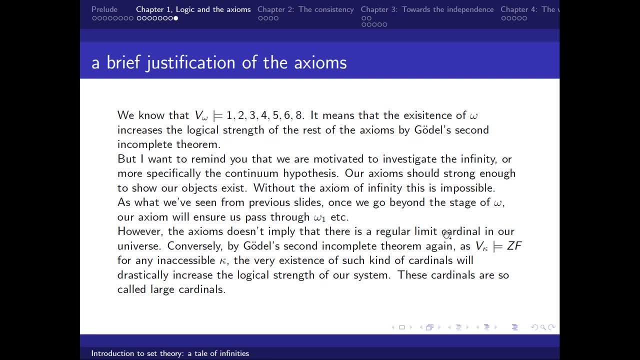 which we also call that weakly inaccessible cardinal. So why the implication doesn't hold By Godot's second incompleteness again. So if there is a regular limit, cardinal, what does that mean? Well, I mean later on, I will just assume GCH holds. 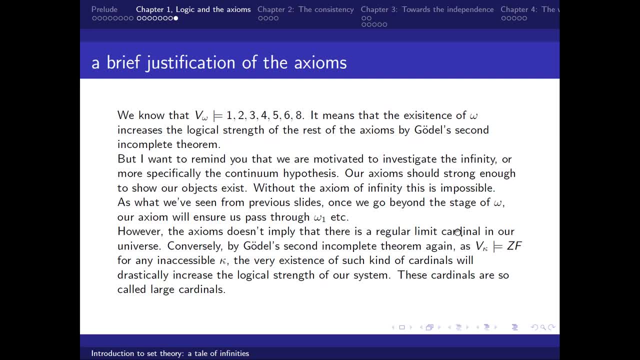 Sorry for that, but let's just assume GCH for this moment. So then Kappa is strongly inaccessible. So if Kappa is a strongly inaccessible cardinal, then we do the same thing: We just cut ourself at the state, at the stage Kappa. 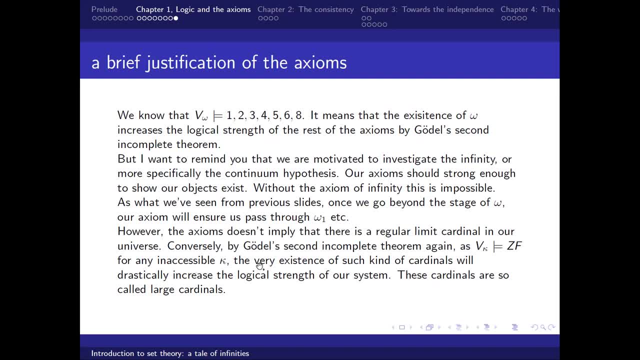 Kappa is going to be a Z-8th model. This time we have the affinity FOR all objects, omega in, because Kappa is inaccessible, way above omega. Okay, So exist the existence of an inaccessible cardinal. just gave you the consistency of ZF, or ZF plus C. 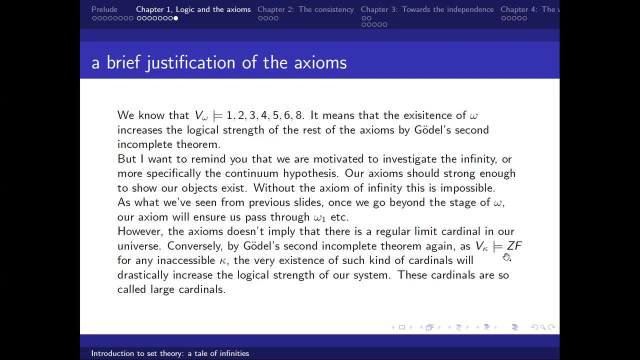 if your universe has C self, So it's going to be stronger than ZFC alone. So that means you cannot prove the existence of that kind of cardinals from ZFC alone. Okay, that's just a brief justification of that For later use. I'm going to mention that. 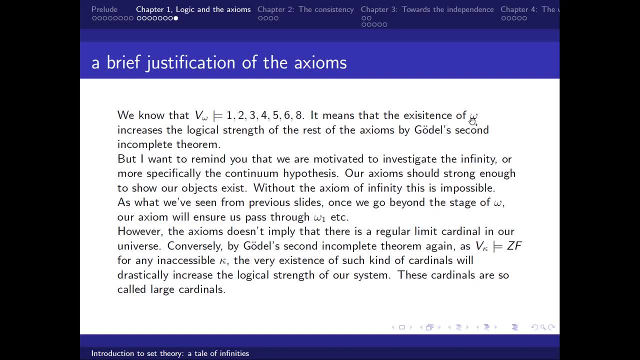 also that omega is also a measurable cardinal. Yeah, but not an uncountable measurable cardinal, So it has a non-principled ultra filter on it. Okay, let me just move on to the. So we finished the naive set theory part. 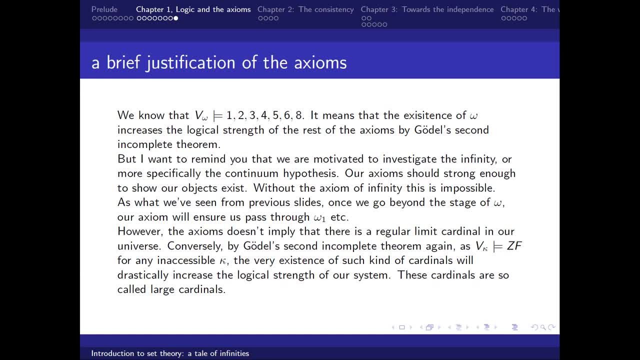 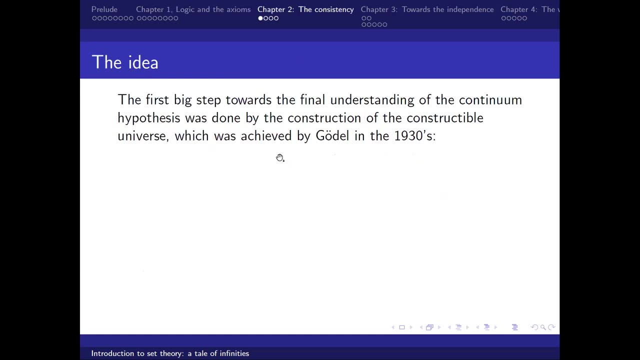 I gave you all the axioms that I need. So let's just move forward for the independency of the continuum hypothesis. So the real processes, the real progress after Cantor's original work was carried out by Goddard in 1930s. 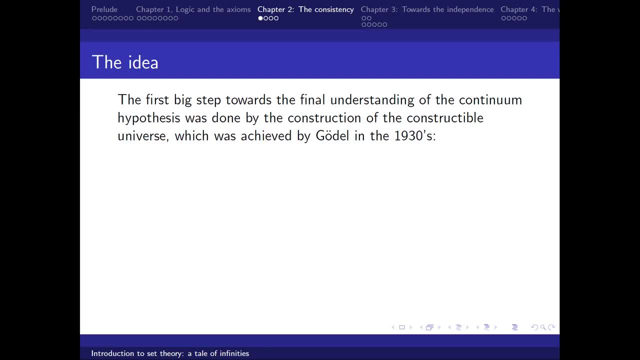 So he just observes that, despite we can't show, CH is true, but it's consistently true. Or in other words, if you have a model of ZFC, he can give you a model which satisfies ZFC plus GCH, based on the model that you gave to him. 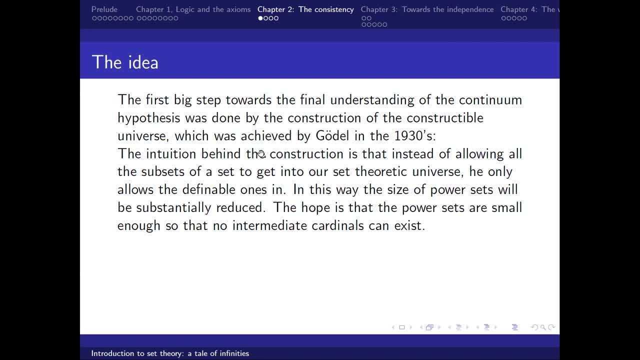 So there are some intuition behind which guides that construction. There are some philosophic motivation behind it, but let me just give you the simplest reason why this is. I mean, why this could work. Okay, so the intuition behind the construction is that 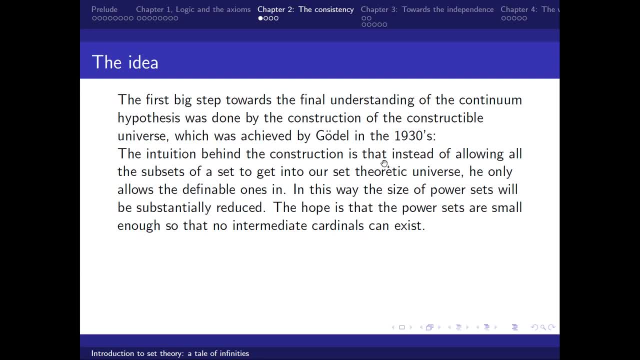 Okay. so the intuition behind the construction is that. Okay. so the intuition behind the construction is that that. so, instead of allowing all the subsets of sets to get into R6 theoretic universe, it only allows the definable ones in. So, in this way, the size of the power sets 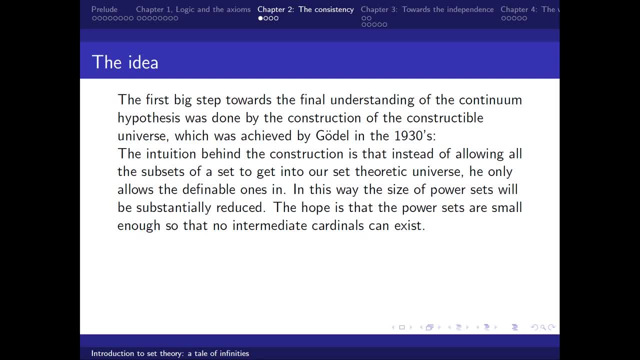 will be substantially reduced because we have- I mean, we rule out- a lot of sets. if a set is not definable, okay, it's not good, we are not going to let it in, And the hope is that in this way, 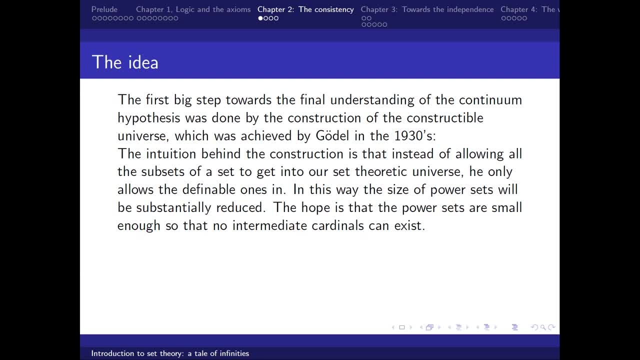 the power set is going to be much smaller. Smaller power sets means that there's more chance that no intermediate cardinals do exist. right, Okay, but there is a trap. I need to warn you that the consistency of the continuum hypothesis is not as simple as just a shrinking power sets. 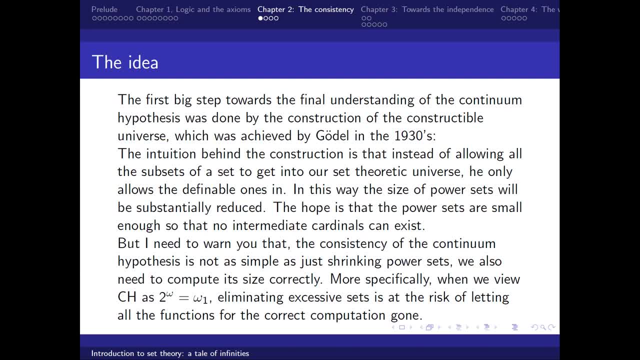 That's what I said before, because we also need to still have the correct function to compute the size of the continuum, Or, more specifically, if we view the continuum hypothesis as the power set of the. so if we assume AC, the real line is real orderable. 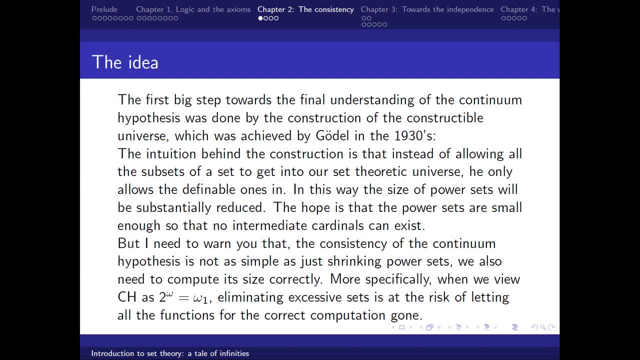 the power set of the nature. numbers is real, orderable. So in this case the continuum hypothesis as the not good, and then, if we substitute the renewing line, be able toandır it to the real evidence. then we said that the continuum hypothesis LinはC單位. 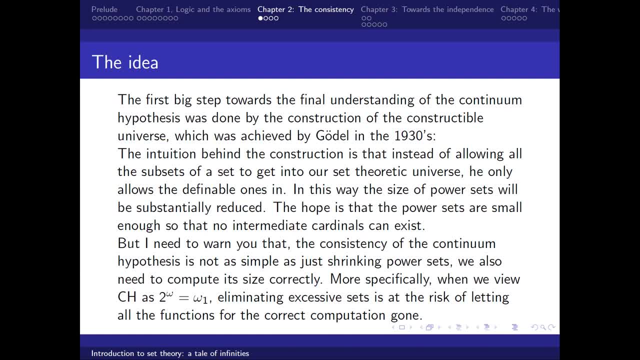 in my Turkide d arrangement will perform the same tasks. right as R6, we were able to determine cell earth dimension. Now I'm just going to add: the astrology alimony hypothesis is equivalent to say that the continuum is the first uncountable cardinal right. 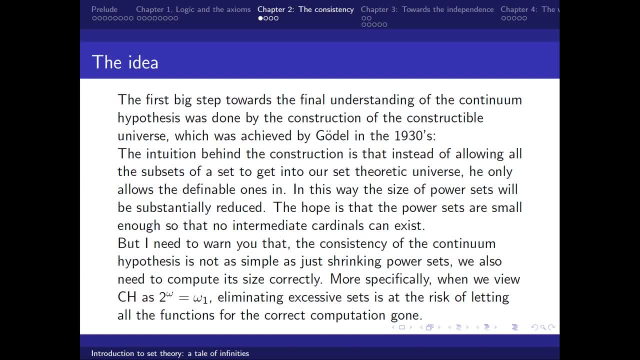 Okay. so if we view this question this way, so if we eliminate too many sets during our construction, so there is a risk that we also get rid of the function that we want for the computation. I will give you some more detailed example about this argument later on. 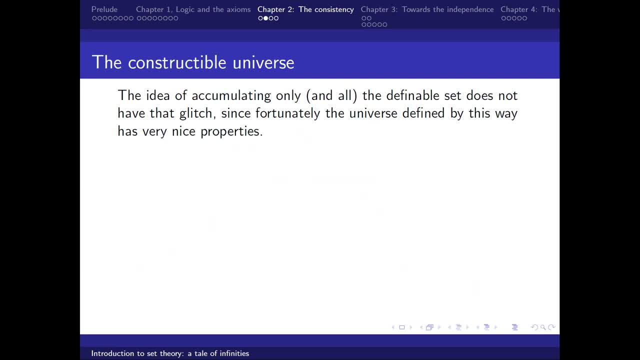 Okay, So the idea of only collect, only collect, only collect, only collecting the definable sets looks like good. it doesn't have that glitch, but it's that's because it's a nice way to define this whole thing. I think it's due to the virtue of the philosophy behind the construction. 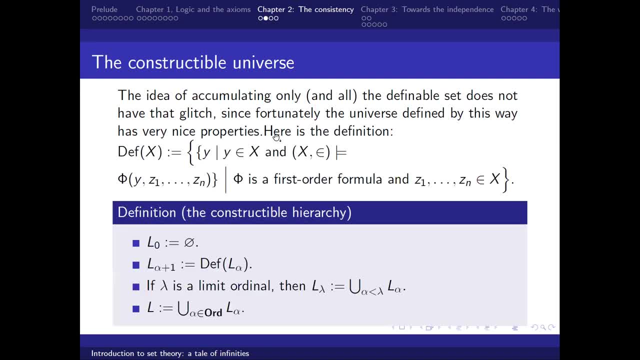 So. so here's the definition. Let me just tell you the sets that we are going to use for the successor stages. So this is basically, says, the collection of the definable subsets of X, namely the set of or y. 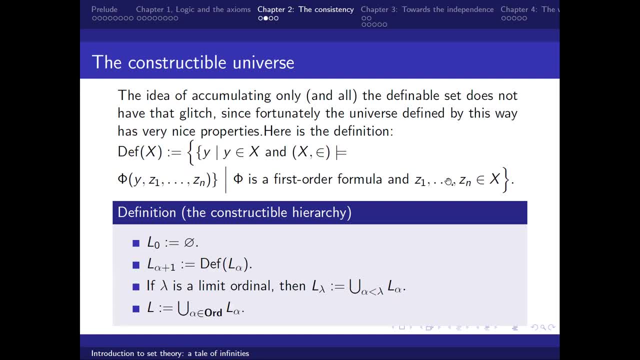 the set of all these collections, the subset of X, which is definable by phi, but we range over all first order formulas with parameters in X. Okay, So this is the definable form. This is the definition of the two sets of the first order formulas. 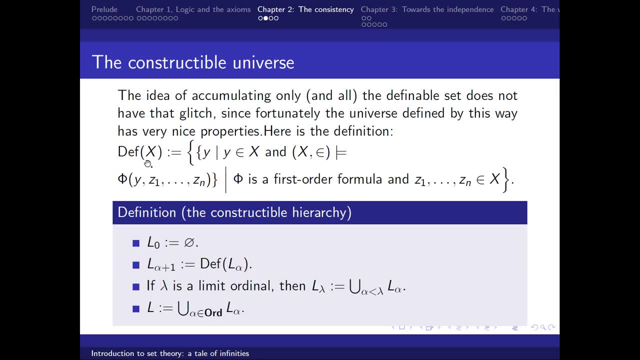 Okay, So this is the definable form. Okay, So this is the definable form, in fact, of x. So here is the definition for the constructable hierarchy. So, again, we start with empty sets. But, you know, instead of taking the full power sets in our construction of cumulative, 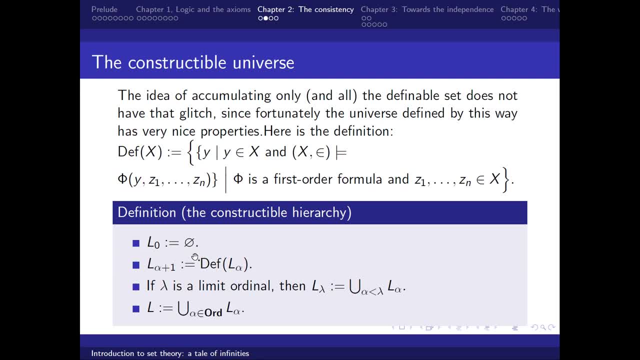 hierarchy. here we only allow all the definable subsets to get in to form the successor stage after a of alpha And for limit ordinal, it's the same. Just take the unions At the constructable universe, it's just the. 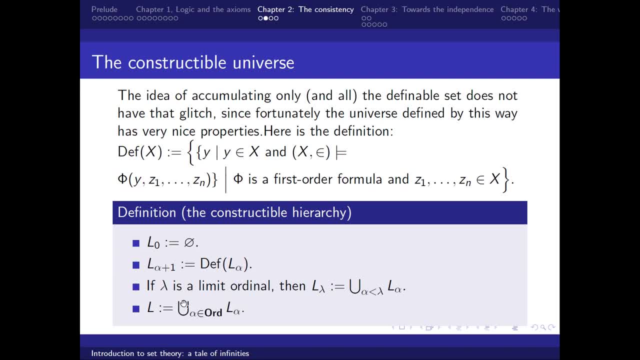 you know, we just take the union of all hierarchies along our ordinal line. okay, So there is one thing that I'm going to use, but I haven't given the definition later on, So this structure can be enriched by some predicate. So let's say: 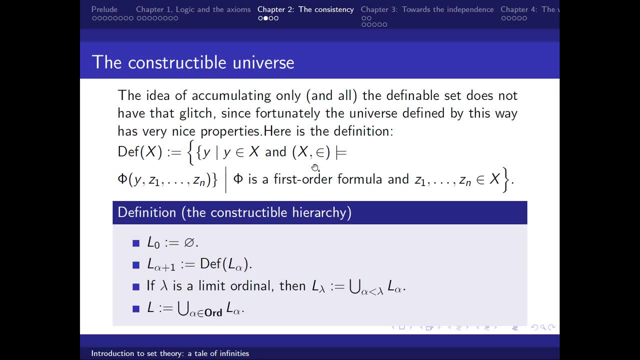 A is a subset, I don't know. I think I can write, I hope you can follow. So fix set. So let me see the definable power set of x relative to some predicate A. The predicate is a subset of x, So 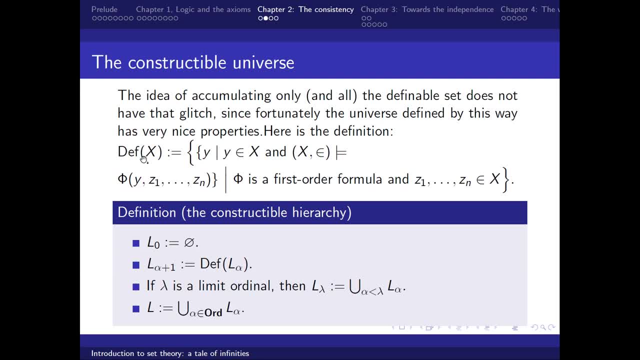 In this scenario we enrich the structure with one more unary predicate A, so the rest of the definitions just stay the same. So A is the first order of formula in the L language with one more unary predicate A. As the structure we construct for the collection, we need to enrich it with the additional predicate. 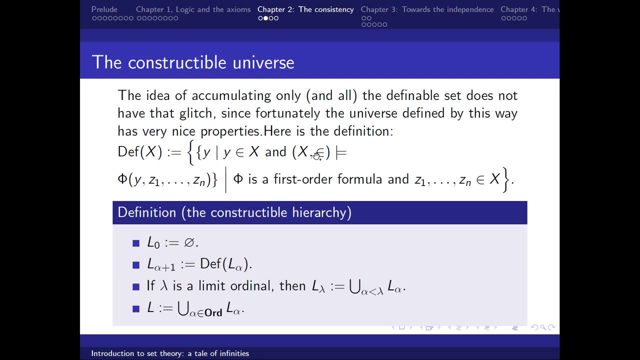 A, That's called the relative-wise. So if we use the enriched definition, that's called the relative-wise constructible universe With one more later: L0A, L, alpha plus 1 of A run a bracket and also L of A bracket. 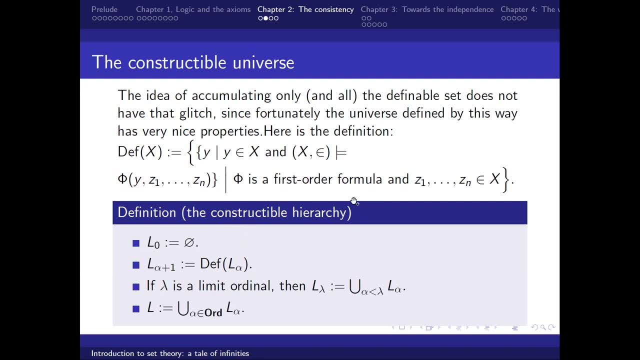 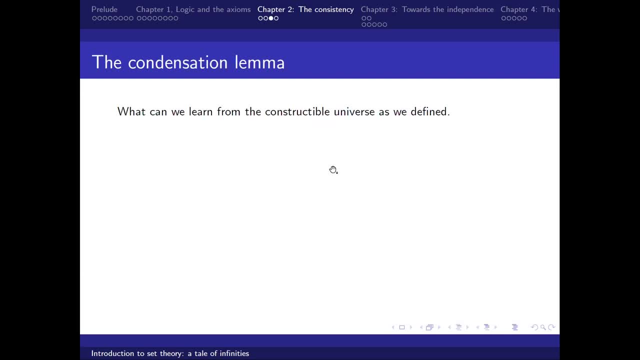 So you will see that later on I'm going to use it during this talk. Okay, what can we learn from the constructible universe as we define it? So, first of all, we can count the size of the constructible hierarchy, sex to the standard. 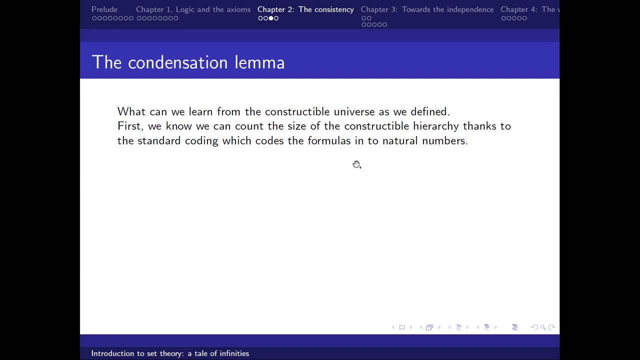 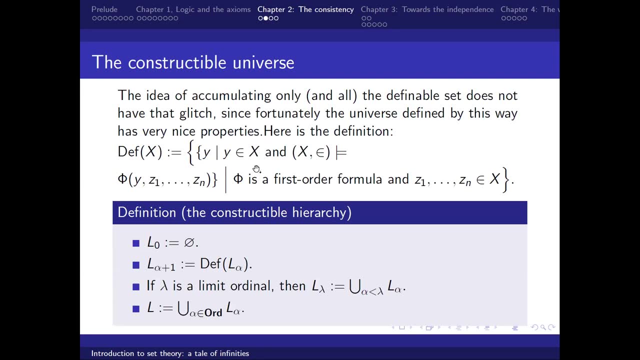 coding, which codes formulas into the natural numbers. So let me go back to the definition. So what's the size of L alpha plus 1? It's exactly the same size as L alpha, because there are only countable many formulas, as the parameters suggest, of the same size of L alpha. 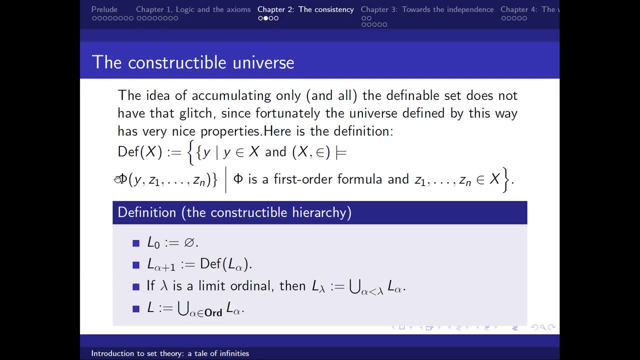 So there are only L alpha size many formulas. Okay, So This is the size of L alpha which allows you to generate definable subsets. So the definable subsets of L alpha is just the same size of L alpha. That's the first thing. 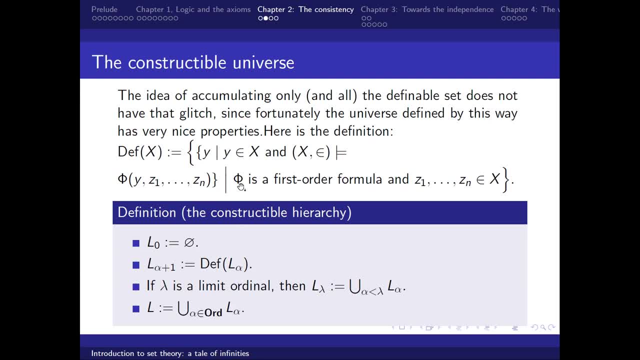 The second thing is that. so by the standard coding the formulas are called as natural numbers. So we can define the. you know, we can define a way of ordering, firstly by the order of the order line, So namely the sets. which enters the constructible hierarchy later on, always comes later in the 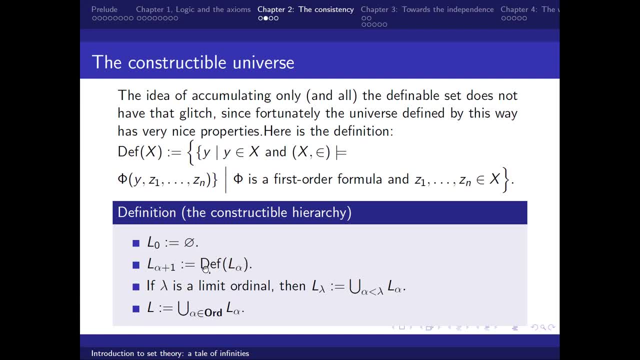 code And with yin one, exactly the definable sets, namely yin L alpha plus one minus L alpha. all the elements can be reordered by the, by the formulas, because again there's a induced order by the natural numbers. 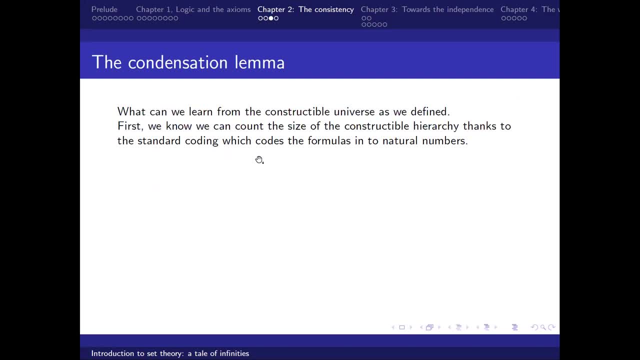 Okay, So that means that's what I said. L kappa is of size, kappa kappa is a cardinal. This is by shown by induction. and secondly, L is the axiom of choice. Okay, Okay, Okay. So that's kind of the model you are going to start with. 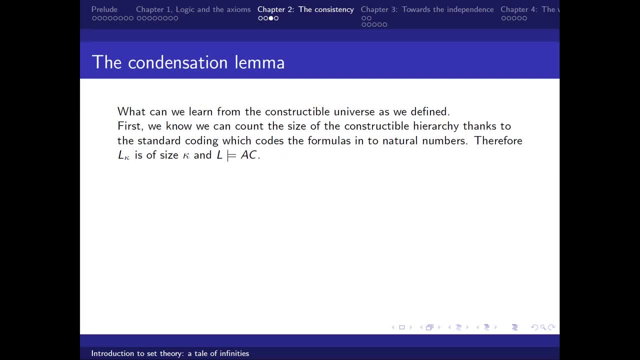 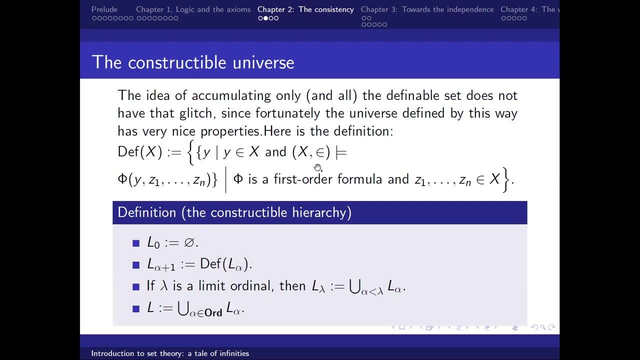 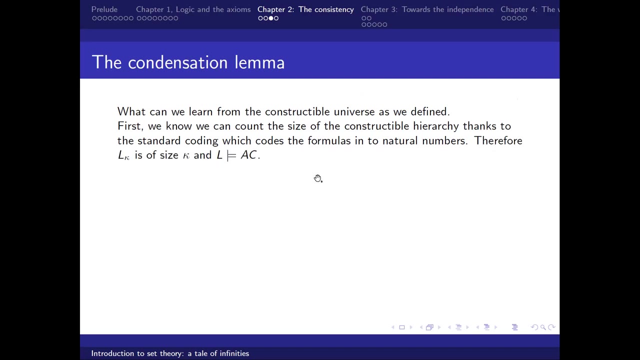 If you start with a model without a choice function, then you do the same construction within that model. you are going to have a model of choice. That's how the you know how we obtain the consistency of the axiom of choice. Okay, 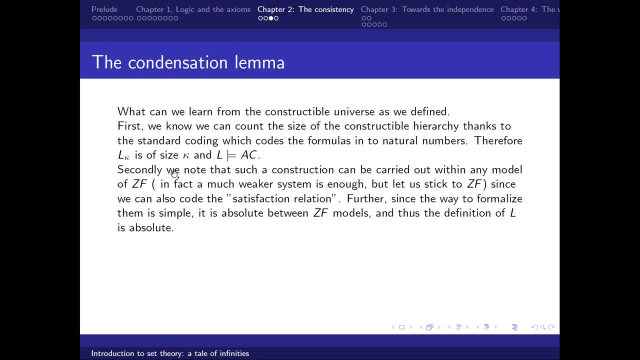 Okay, Or what you're after. So you have single numbers, right? Yeah, Simple questions are used for, you know, flexible, kind of unconscious� questions. Okay, Mm-hmm, And by an argument though you're going to be able to use. I don't know, I guess you. 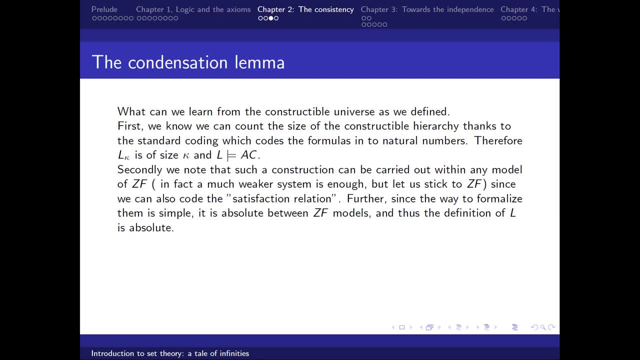 can ask yourself some questions. Uh-oh, Brilliant. Yes, the F, Since not only the formulas can be coded into natural numbers, the satisfactory relations can also be coded into subset of natural numbers. So you do the coding within a ZF model. 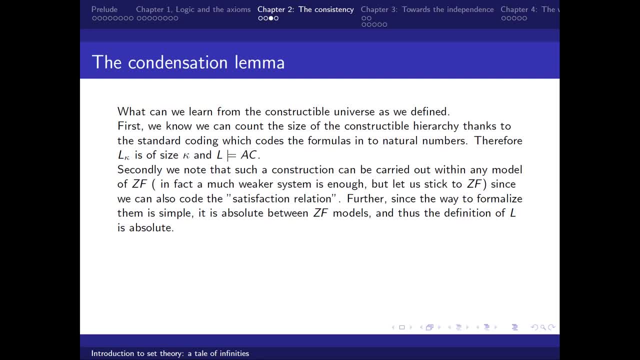 Okay, that's all. But one more important fact is that the way to formalize this set-faction relation, the way to define what a formula is, is actually very simple in the sense of logic. It's actually delta one one complicity. 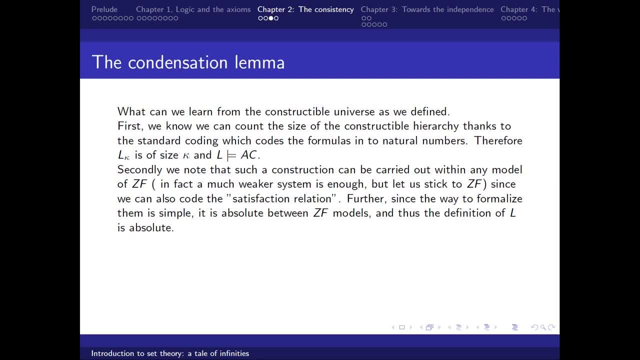 That means it's absolute within the F models And hence L is absolute. That means whenever you have an inner model M of way L in the sense of M, namely you construct L inside M- you are going to get the same thing when you construct L inside way. 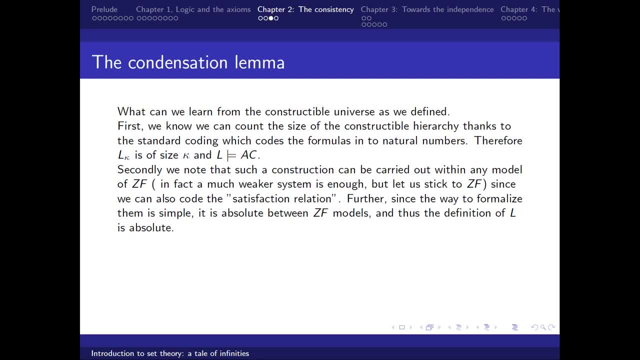 So this absoluteness also gives you that L is the minimal model, minimal inner model of the F. So okay, So this property is just a paved way to the following theorems called condensation. So for every limit, all you know, delta. 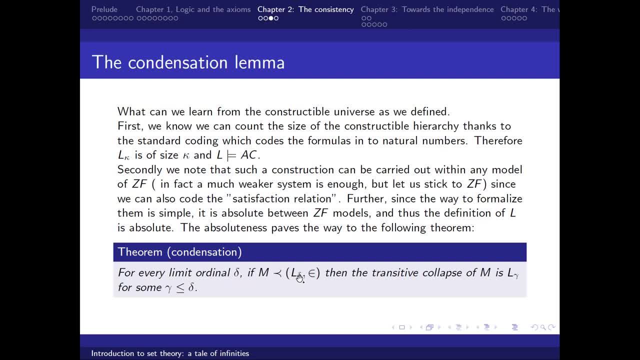 So L delta is going to satisfy enough segment of the F which enables you. So it's a much weaker system. It's not much weaker, but it's a weaker. It could be a weaker system for the F, but that's enough. 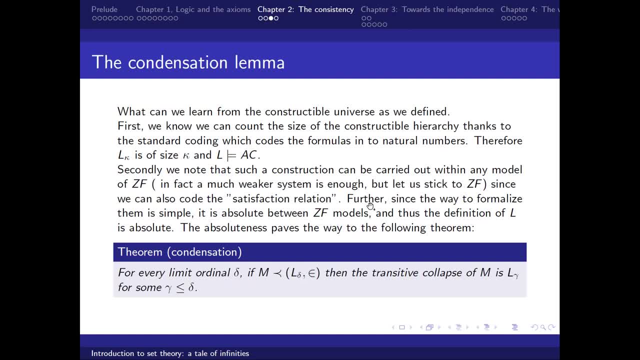 But if that's enough for the construction of L, so for every limit, all you know delta. if M is an elementary substructure of L delta, then the transitive collapse of M is L gamma of some gamma less than or equal to delta, of course. 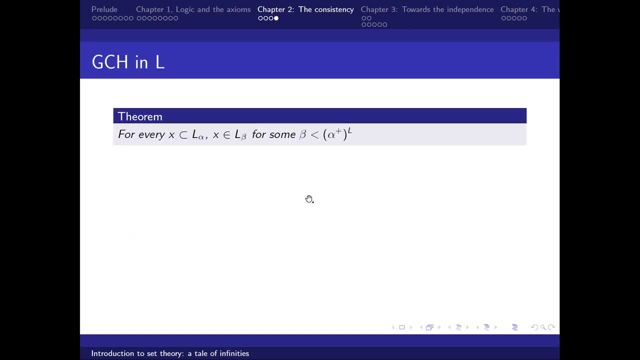 So that's called condensation. So with the help of that condensation lemma. so here is the theorem which will eventually give you the GSI: H holds in L, So which says that if X is a subset of L alpha, then X must be accept into the constructable hierarchy before. 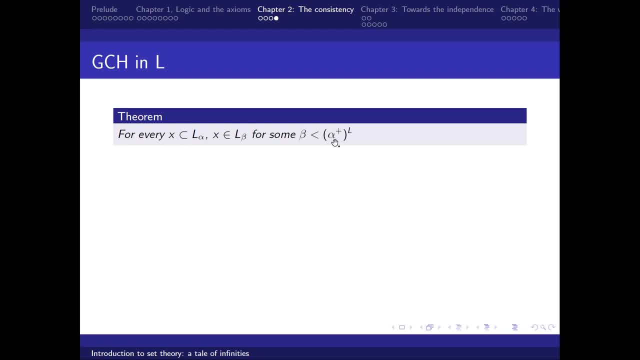 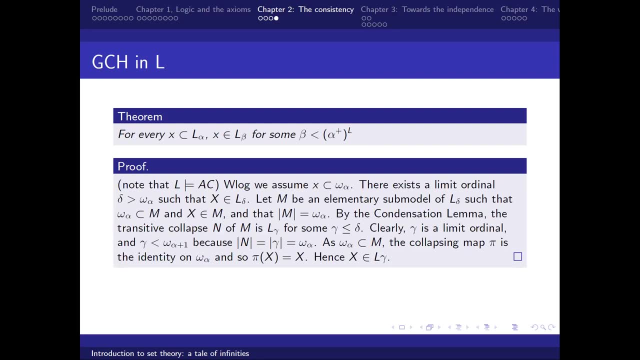 the stage of alpha, plus of course, in the sense of L. So here is the proof. So note that L is a model of axiom of choice, as what I showed you. So, without loose of generality, we can assume that X is a subset of ordinal. 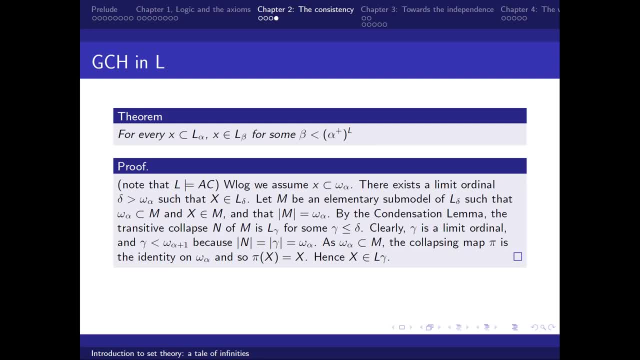 Let's say omega alpha. Fine, Okay, We just choose the limit of L. There is one, there is a limit: ordinal delta greater than omega alpha. so that X is in because X is in L, right? So yeah, I think here's a typo. I think should be capital letters: X, okay. 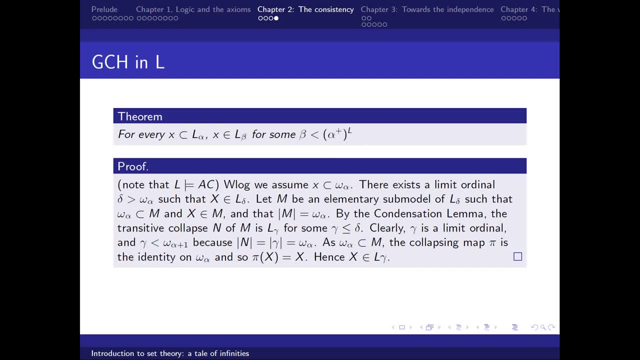 Okay, So okay. now takes elementary substructure of L delta, so that it contains omega alpha, and X is also in that M. But by the standard Lohmann time-scaled theorem M is of size omega alpha without any problem. 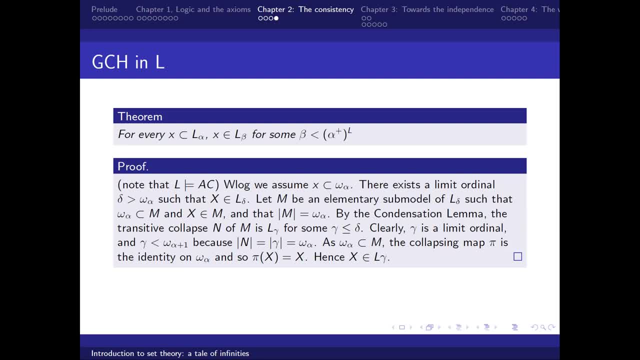 but by the standard Lohmann time-scaled theorem M is of size omega alpha without any problem. but by the standard Lohmann time-scaled theorem M is of size omega alpha without any problem. now we are going to apply the compensation lemma to that. 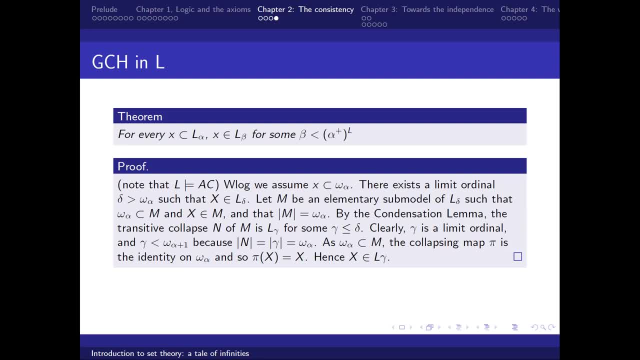 which shows that if we trust the collapse, our M to get an N, N is going to be L, gamma for some gamma, And again trivially by the. there is a formula which says that the universe is limit or successor. I mean, that's trivially true that gamma must be a limit ordinal. 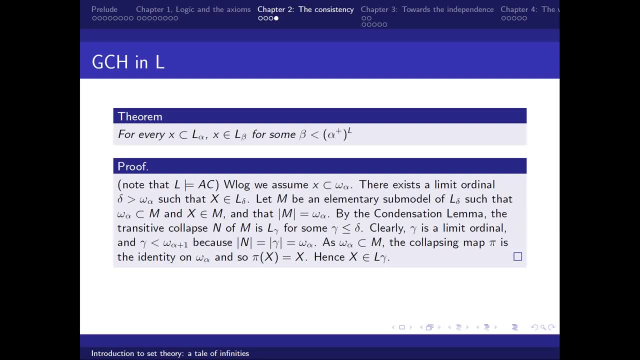 this is implied by the elementarity of the L, delta is. delta is the limit ordinal. So gamma is the limit ordinal. but gamma also have to be of size strictly less than omega alpha plus, which is omega alpha plus one, because the size of the 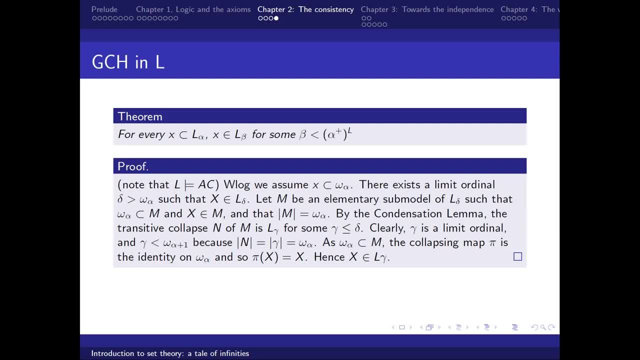 the model is of size: omega alpha. Note that M is of size: omega alpha. you do the drastic collapses, such as the bijection, but we have the omega alpha as a set, which is including our M. that means the collapse function, do not. 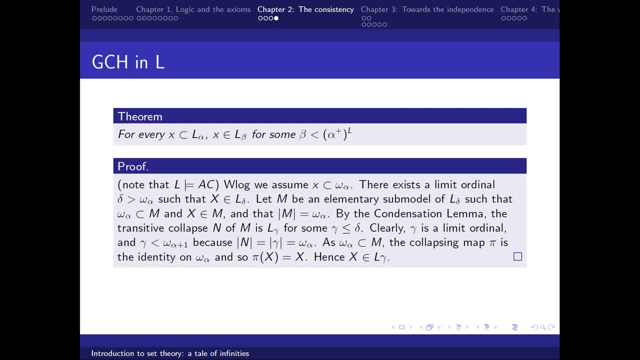 I mean do not collapse at all or say, identity below that part means that X under this collapse map is not moved. So the collapse is going to map X to X itself. And okay, so then this gives you that X is in X. 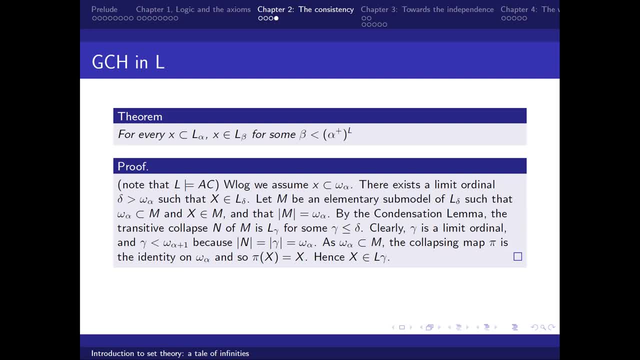 and then this gives you that X is in Y, and then this gives you that X is in Y, and then this gives you that X is in L gamma as what we want, right? So X is in some L gamma. gamma is the same omega, alpha plus. 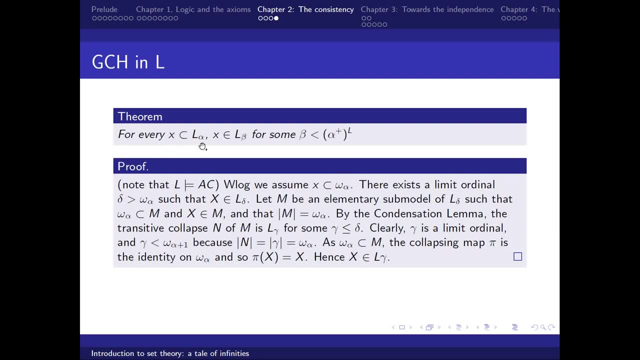 So for any X in L, omega alpha, it's going to enter the constructive hierarchy before the stage of omega. Okay, Omega alpha plus in L. So now as a corollary. so if L is an L cardinal, again the, so L thinks the positive alpha is just the. 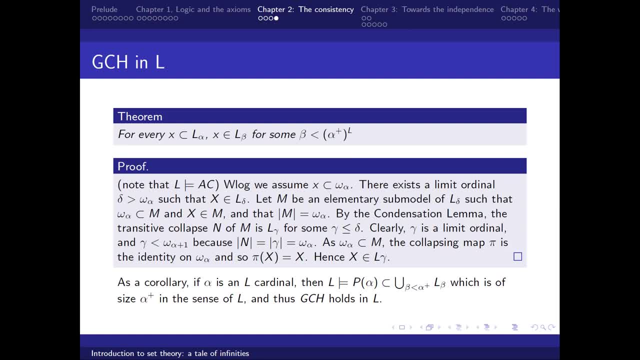 you know, the union of the, the constructible hierarchies before the stage of alpha plus. This is what this theorem tells us, But which this set, this union set, is going to be of size alpha plus, because it's alpha plus many sets of size, actually alpha. 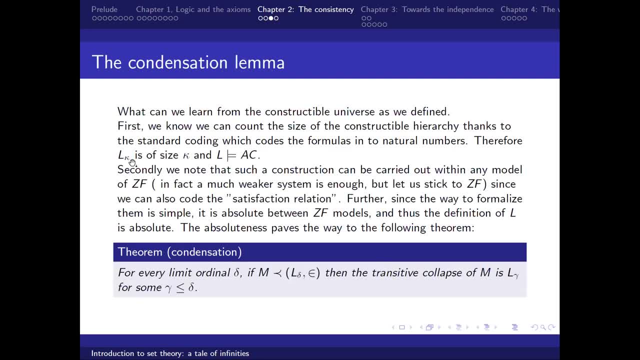 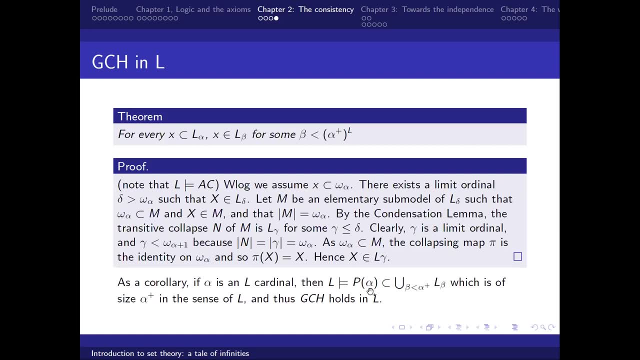 as what we've seen Here right. So that means L thinks the positive alpha is contained in some set of size alpha plus that apply to all the cardinals. So GCH essentially holds in L. Yeah, So I think I. I went a little bit faster than I thought to be. 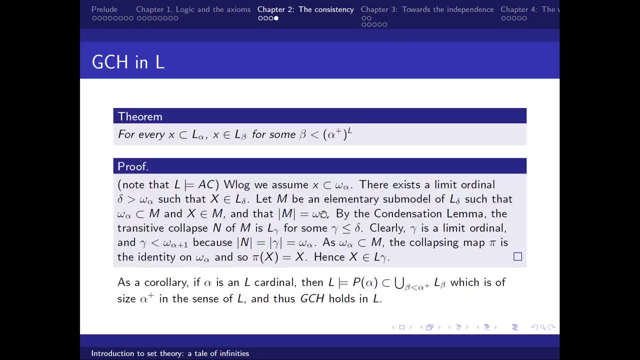 I don't want to enter the independence proof today, So can we finish now or you want to go ahead? I suppose it depends on the audience Or just the leave the rest of the time. Yeah, Yeah, Yeah, Yeah Yeah. 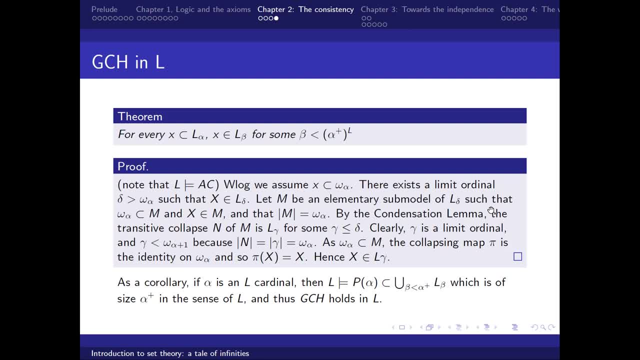 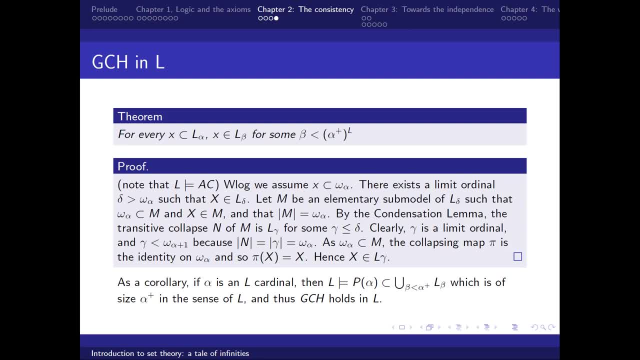 Okay, Yeah, I think Yeah, Because I think I went a little bit faster than I thought. I hope that everyone of you can follow. So just time for questions. okay, does anyone have any questions? yeah, it seems like no questions, uh, so far. um. 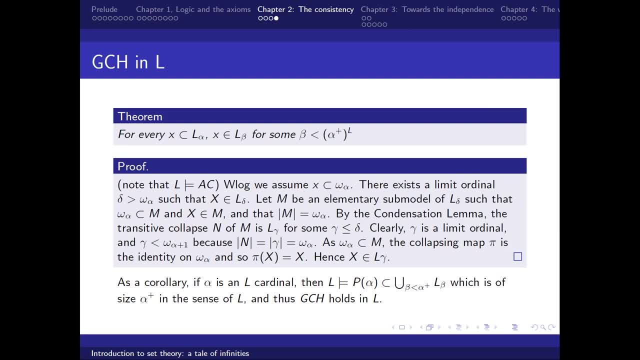 but i guess, uh, if there's any further questions, they can ask you again in your next session, okay, or do you want me to move forward? i mean, i think there's a lot of things. i mean, if you are not familiar with, say, theory, it's already a lot of new things to you. so 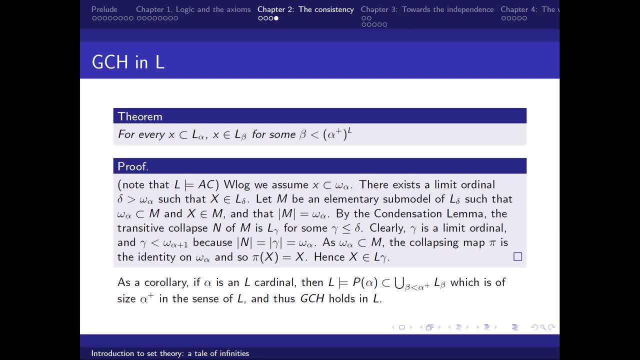 yeah, i mean uh, to me definitely yes, because, um, i'm not a mathematician, i'm a physicist, so, uh, i think a lot of this for the first time, uh, but for for the the rest in the audience, uh, i, most of them should be mathematicians, i think. 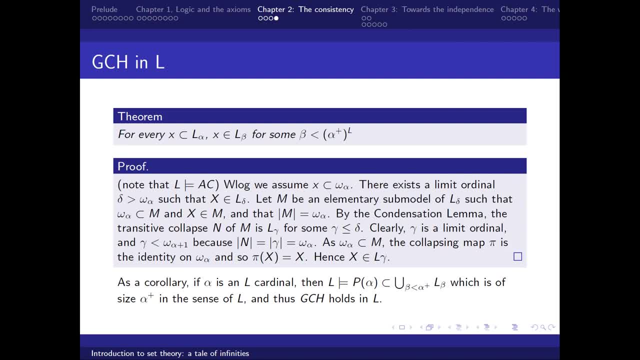 so let's just stop here. i will leave time for you to digest the thing that i had talked. yeah, okay, yeah, that sounds uh, yeah, i think that's fine. um so okay, yeah, thank you, uh, dr yan, for the nice uh introduction and uh lecture. so, um, yeah, so i suppose that should be. 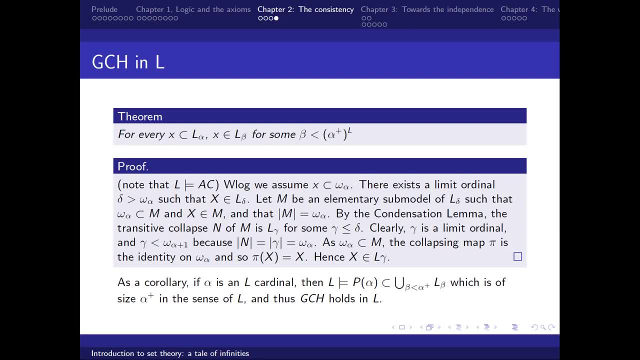 all for today. um, for uh administratively, i suppose uh the next, i should mention the next uh session will be the lecture two for uh- introductory model theory- is on uh february 12th uh, 1 am to 3 am utc. uh, it should be 9, 9 am malaysian time, so it's on february 12, 1 am to 3 am utc. 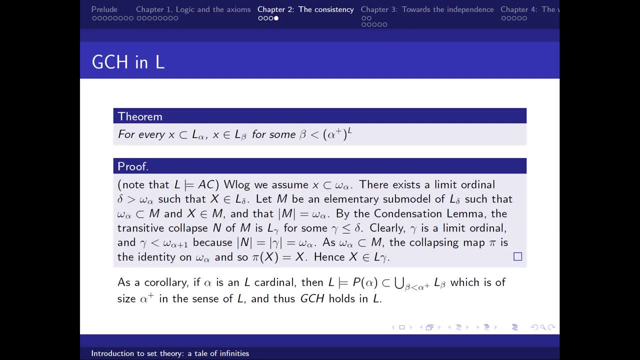 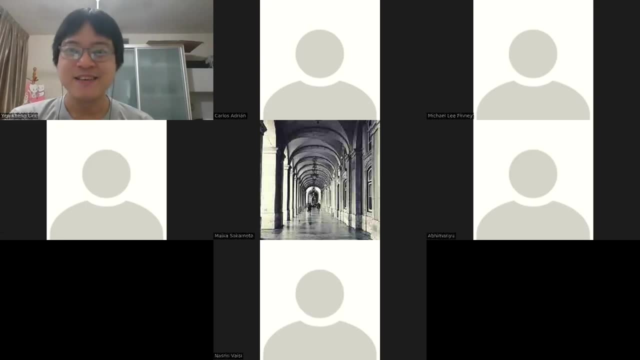 in any case, you can check your google calendar. that automatically convert converts it to your local time, um, so with that, i think that is all for today. so thank you very much, uh, jachen, and thanks to everyone for joining. yeah, so bye, everyone. nice to see you guys, and see you guys in the next session. bye, good night, yeah, good night, are you. uh, are you? 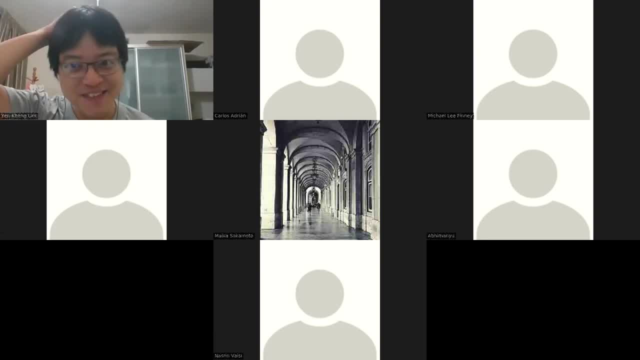 in? uh where? which time zone are you in now? yeah, i'm in uk's uh- greenwich- meantime, so now it's 5: 39 pm, so for me it's evening by definition, but for you it's night. sorry for hold you on q so late. oh no, it's okay. yeah, we're prepared. yeah, so it's like what? 1: 30 am here in malinda. 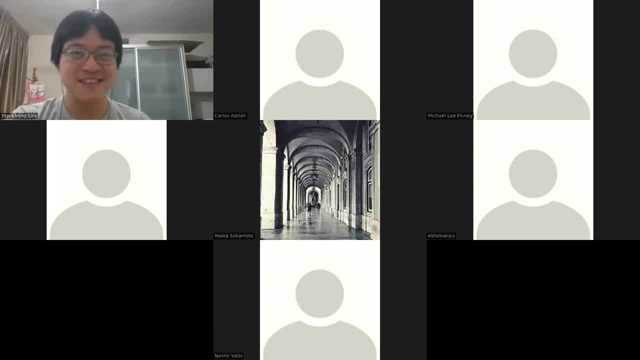 okay. so yeah, thank you very much. thanks again. goodbye, everyone, bye.